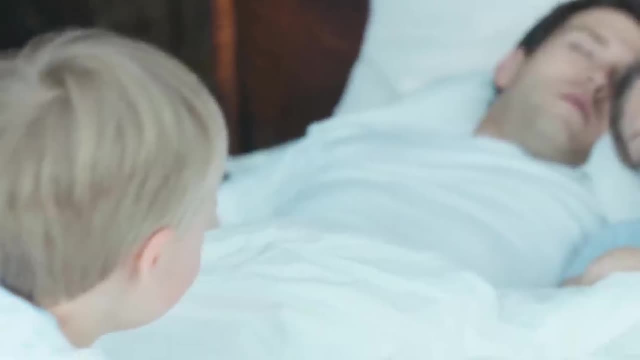 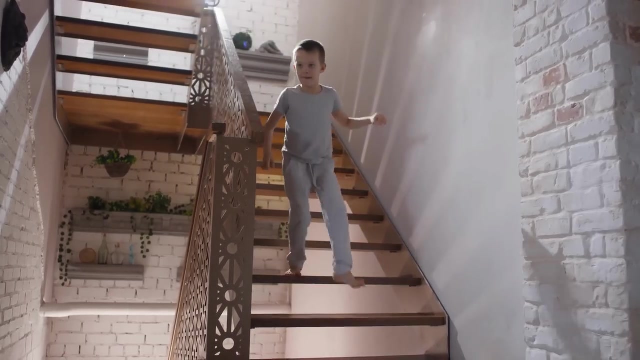 downstairs. I quickly ran to my parents and shook them back and forth while saying: it's Christmas, it's Christmas, but like in a kid's voice. As I made my way down the stairs, I was greeted with exactly what I had envisioned the night before: A decorated tree surrounded by 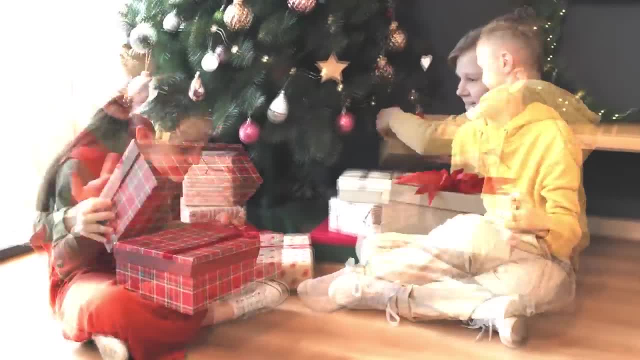 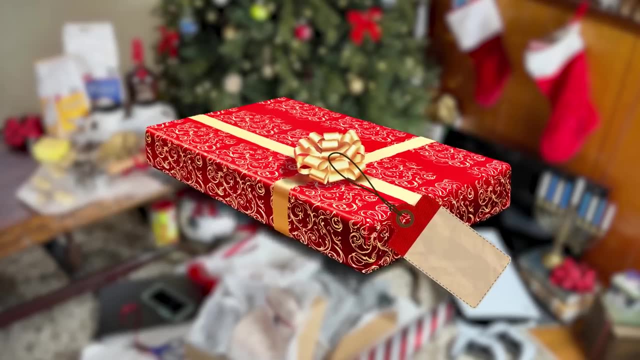 presents of all different colors and sizes. In typical fashion, my sister and I took turns opening gifts until I got to my last one. It was a box with bright red gift wrap and a tag that said: To Cole From Santa. When I unwrapped the first quarter of it, I immediately knew what it was. 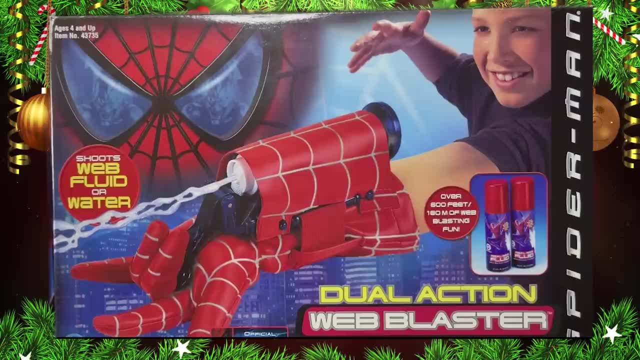 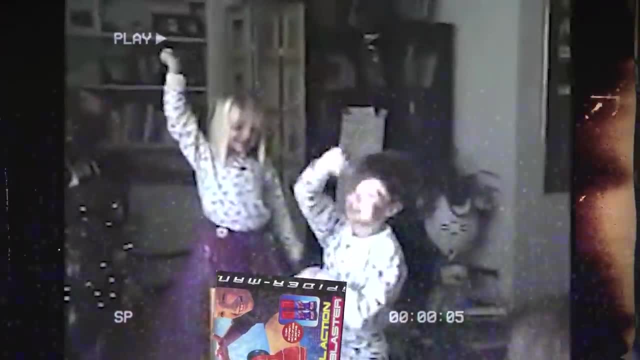 The Spider-Man dual action web blaster that I had been wishing for the entire year. My parents had their old camcorder out and were filming my screams as I stood up and started pacing back and forth. In that moment, it was everything I could have hoped for. 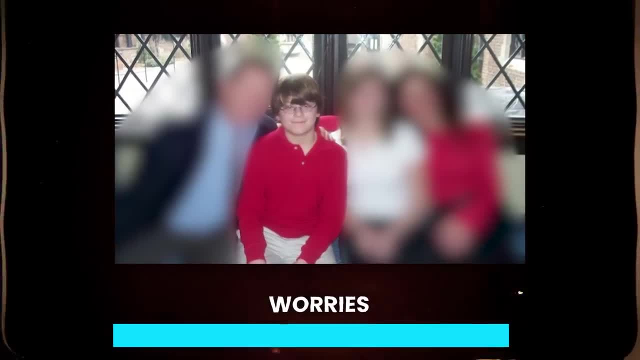 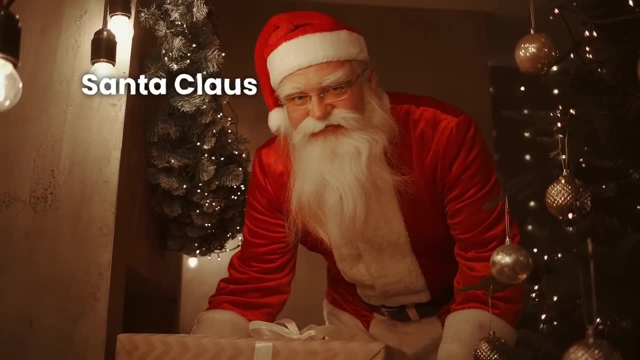 The worries I had back then, in a time where the internet was basically non-existent and the culture of America was so vastly different, were little to none. I trusted in the belief of a man named Santa Claus, and no one could tell me otherwise. All that I was surrounded with were 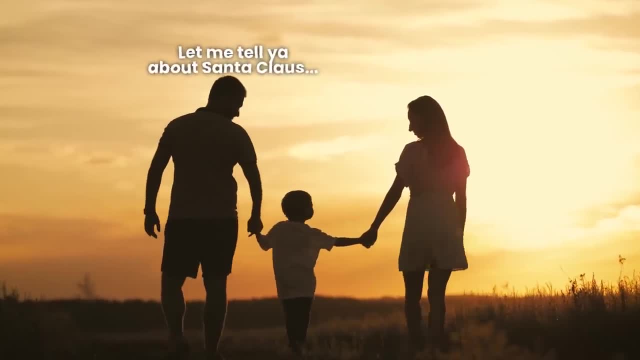 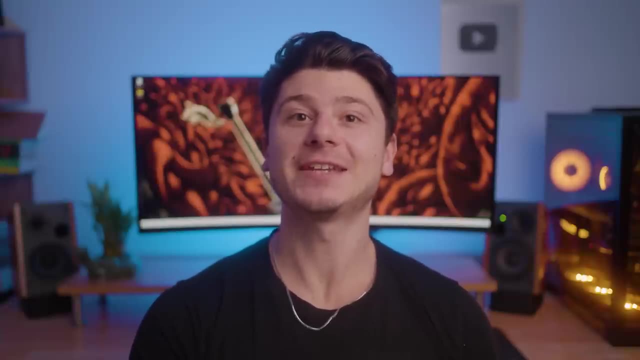 other kids my age or parents who were also dedicated to telling me about the magic of Christmas Day. Now, the reason I bring up this story is because I think that many adults and teenagers have gotten back to the state in which they were born, And I think that's why I'm so. 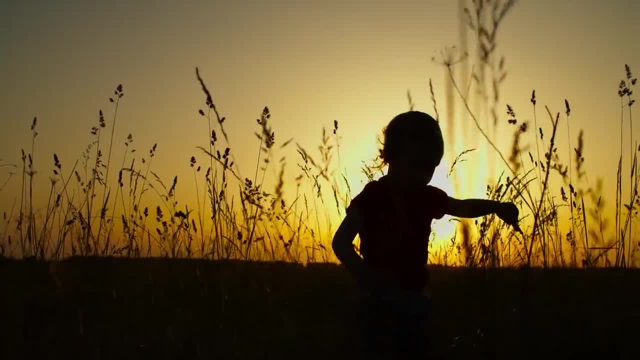 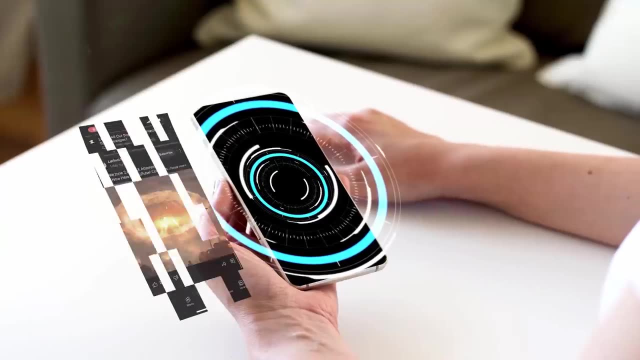 proud to be a part of this story. But instead of that lack of critical thinking coming from their brain, not being fully developed yet and not having the ability to question their authority, like me during that time, it is now because we have a thousand different belief systems that 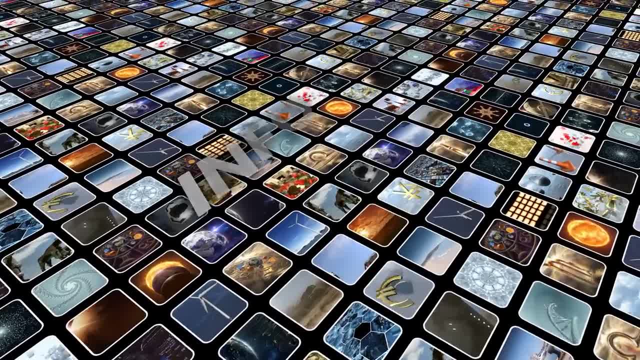 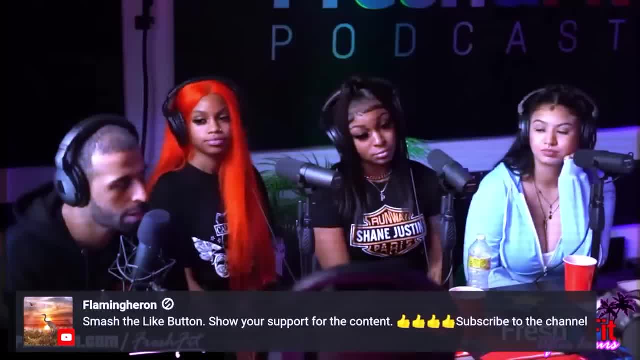 can be easily accessed at our fingertips and we are being faced with information overload. The fighting in Ukraine continues. Collectible f***ing sneakers. You're not being polite, to the pronouns. Most modern day women don't offer much value. One theme that is commonly brought up: 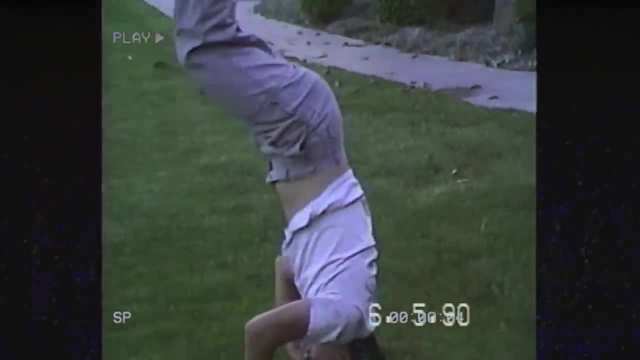 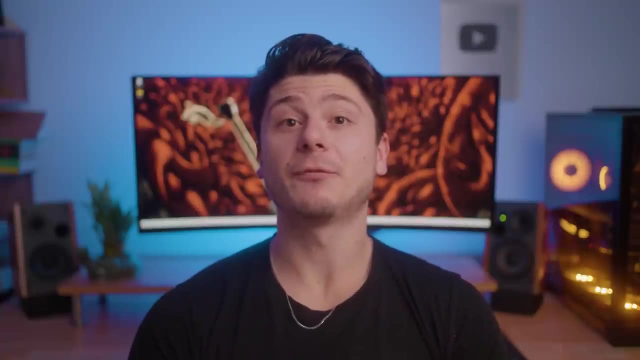 amongst people who grew up in the 90s or early 2000s, whether they were a kid or an adult, is this sense of awe and wonder. There was space to breathe and in many different cases, you were the one that had to figure out the best course of action towards thinking about something. 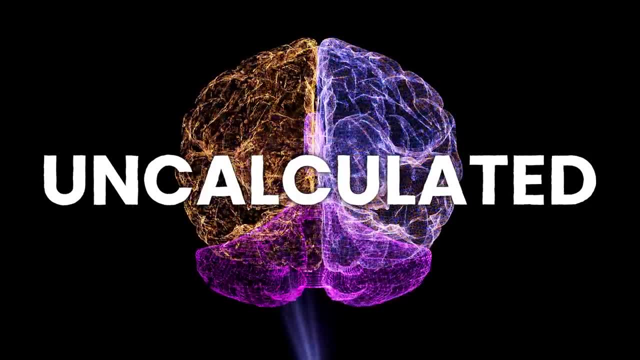 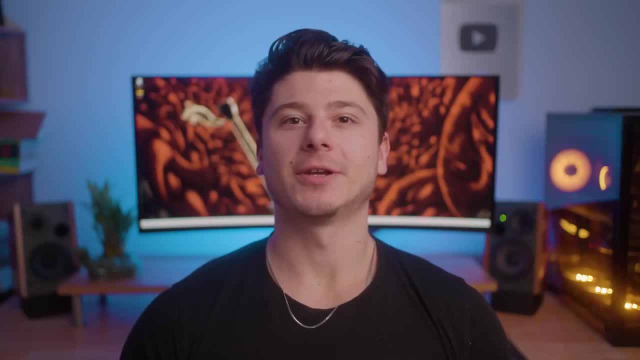 or doing something. In other words, life was more uncalculated, and I think this is massively important towards developing better critical thinking skills. Think of how new and exciting everything felt during this time period: All of these technologies like the internet. 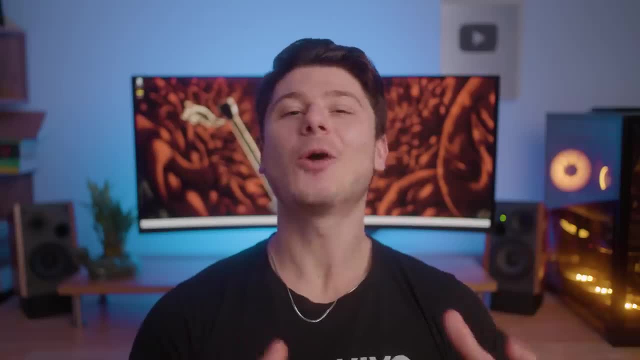 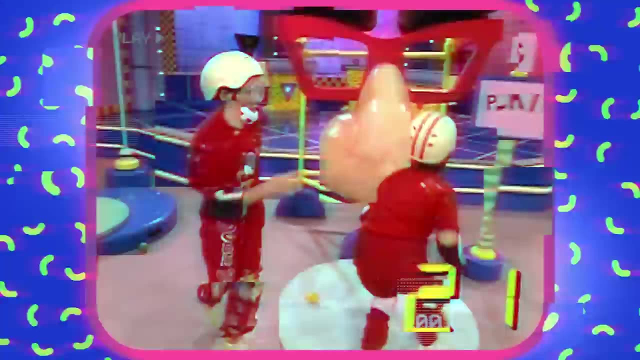 cell phones and more television networks were just emerging. I remember how many TV shows there were that I watched that felt more like an experiment rather than a show that was trying to do as good as possible. When's the last time we had a show like Double Dare, where kids 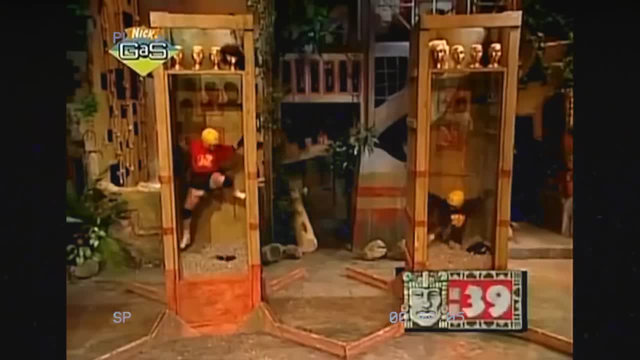 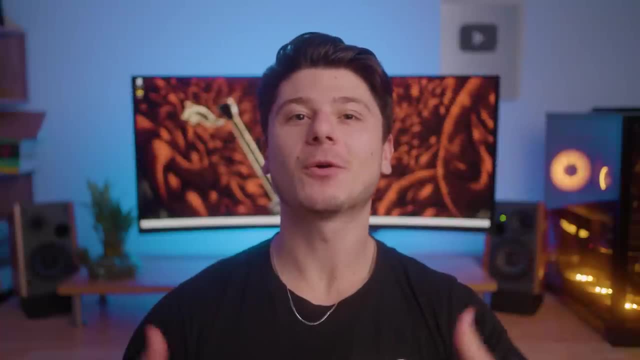 had to grab a flag out of a bunch of goo in a massive nose. Or Legends of the Hidden Temple where they had to climb between two walls to put a wig on a mannequin's head. I don't know. it just felt like each new way of presenting or expressing something felt more inventive. 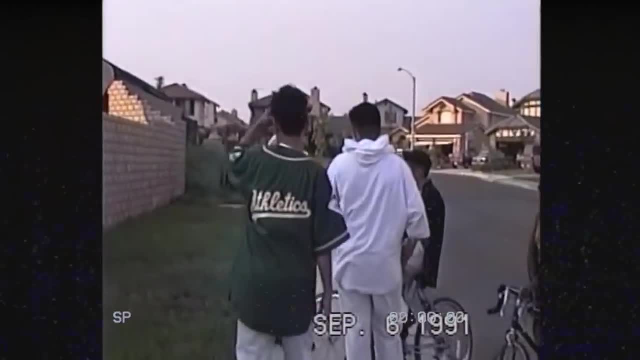 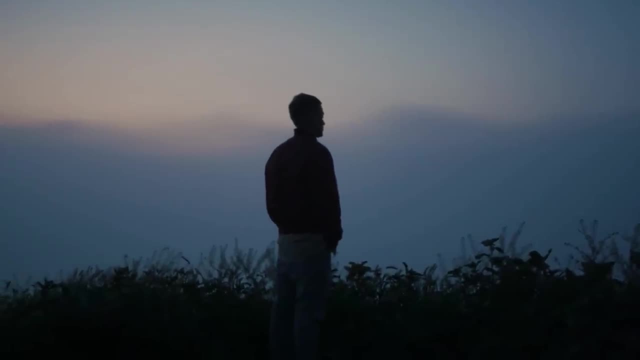 rather than so, bound by a preconditioned rule, And other people's opinions other than the people that you surrounded yourself with in real life were much more scary, Which allowed the individual more of a chance to form their own opinion. But ever since the 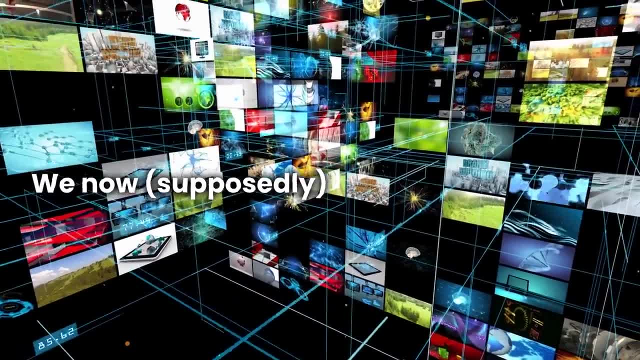 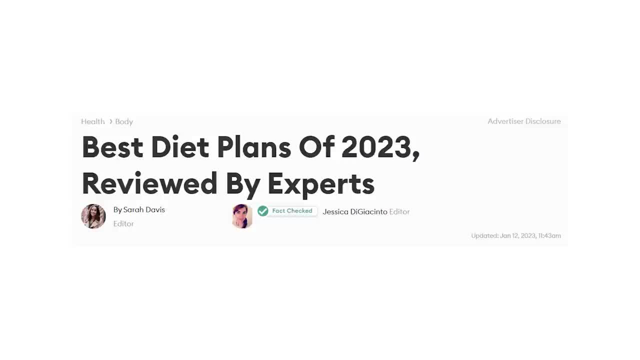 internet became the number one source for all information. we now supposedly have all the answers. Want your business to do as good as possible? Run it exactly like this. Want to figure out the best diet? Just eat these things. You want to be happier? All you gotta do is this. 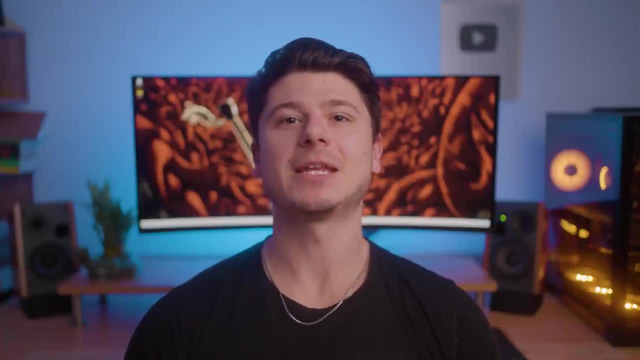 Of course, having more answers rather than less is extremely beneficial in many cases, like diet, exercise, sleep or how to unclog your sink, but there has to be some sort of downside to not being able to figure out things on your own. 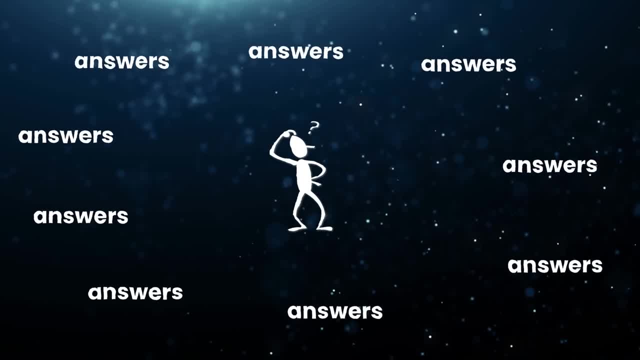 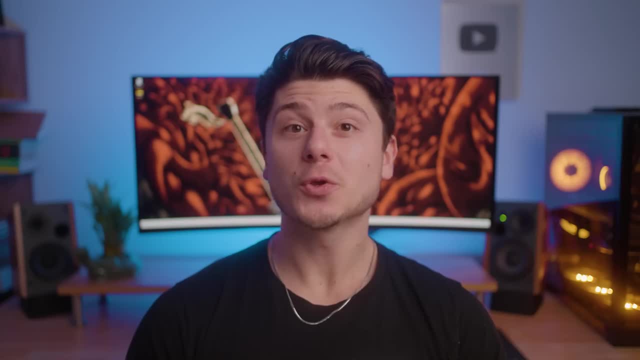 and having that room to wonder. And that downside, I believe, is a lack of deep critical thinking. that comes only when one doesn't always have an answer or think they have an answer to everything Now, before you can even conceive an opinion on something, your opinion has already. 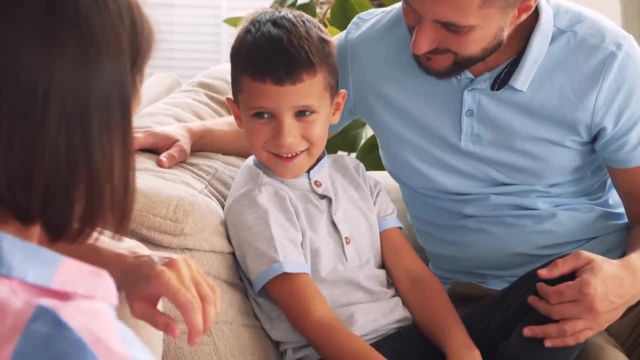 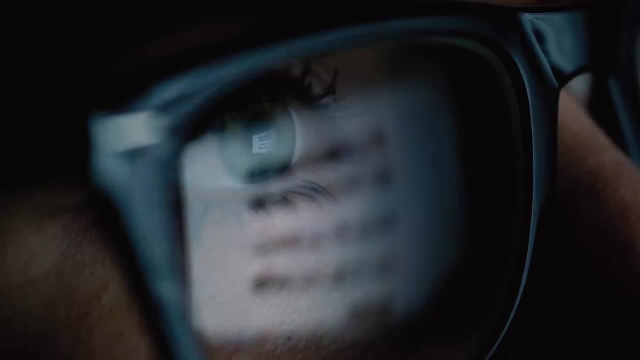 been decided for you by the internet. Just like how your parents tell you who Santa Claus is and why he exists as a kid, the internet is like that parent that tells you their own viewpoint on the world and doesn't give you any room to question it. And it seems so counterintuitive because 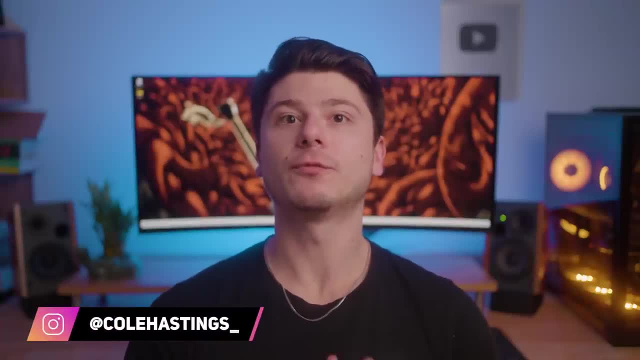 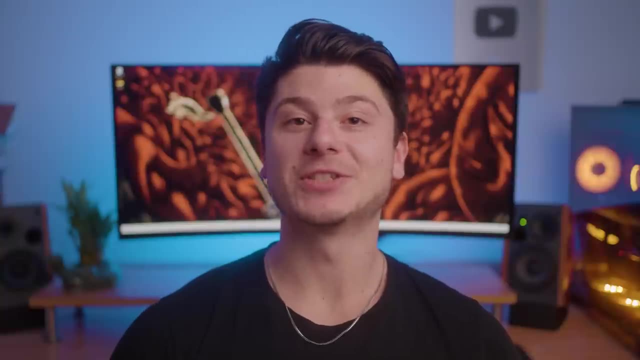 if we had all the information and every single viewpoint we need in order to form an objective opinion, our ability to form rational critical thought would increase, But I think for many people it's been the exact opposite, Because it's so much easier to get the immediate answer. 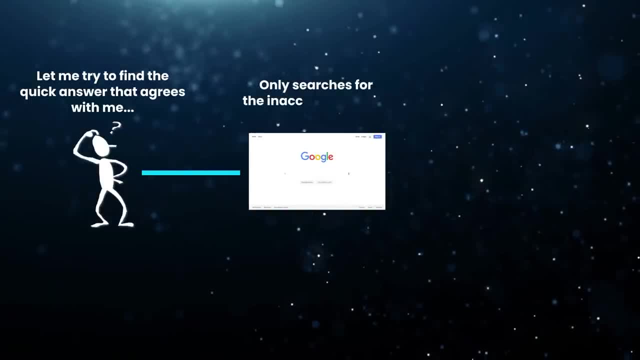 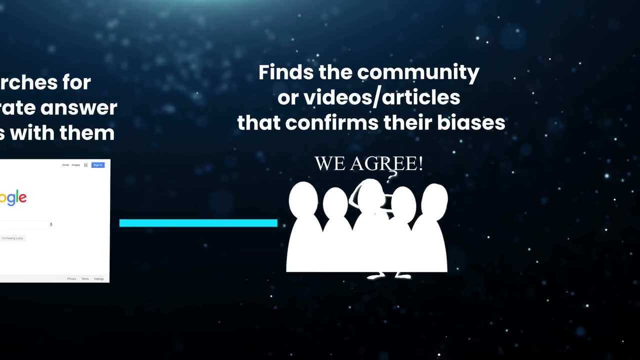 your brain is looking for online, which, in most cases, isn't the critically thought out answer. you have more confirmation than ever that your opinion is the right one, So you really don't need to use the brainpower required to believe in anything else other than what's presented. 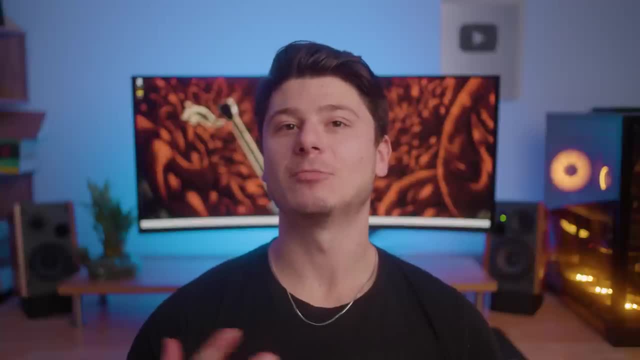 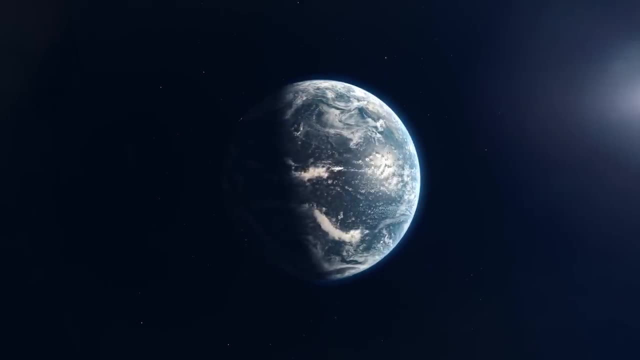 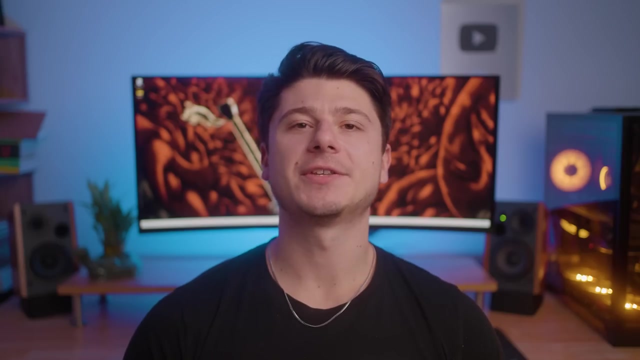 in your internet bubble, But I'll explain that in more detail later. I also think that, because there was much more space for people to think for themselves, the world also moved much slower in general, And what's now taken its place is an extremely capitalistic society that thrives on hyper-competition. Now competition has 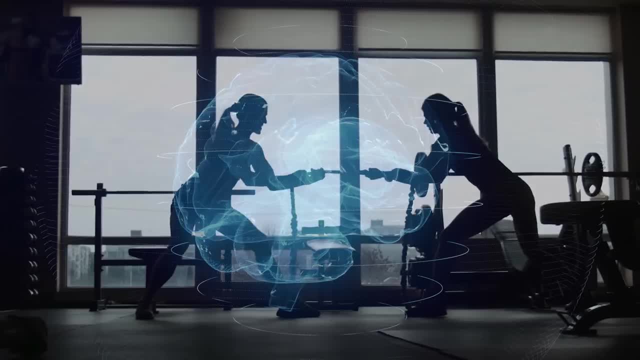 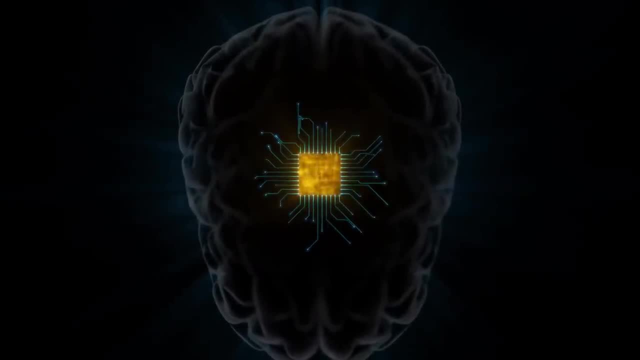 always been prevalent since humans have been around. We are wired to compete with each other over resources, relationships and status. in order to survive, The more animalistic parts of our brain form to ensure we would continue to progress and reproduce, and that's a good thing. But sometimes 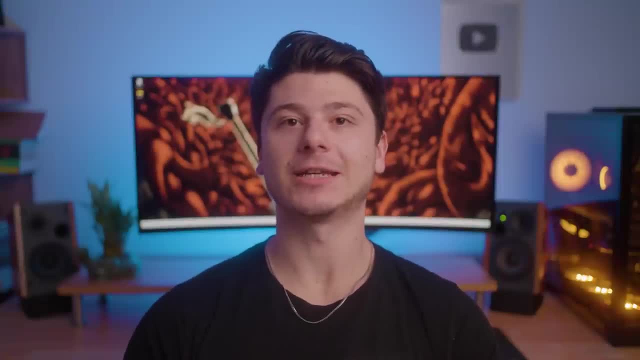 too much of what we do is not enough, And that's why we have to think about how we can move forward, And I think that's what we are seeing now, In a world where you have practically zero time to situate yourself with your job or 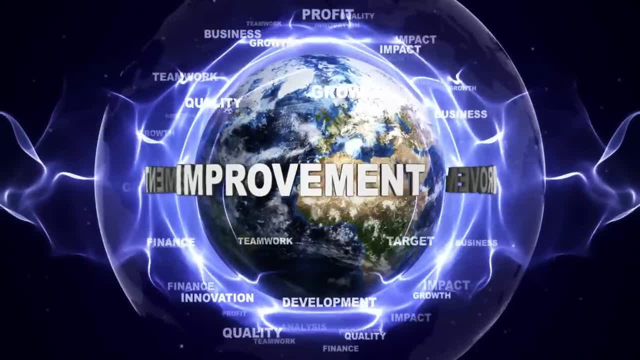 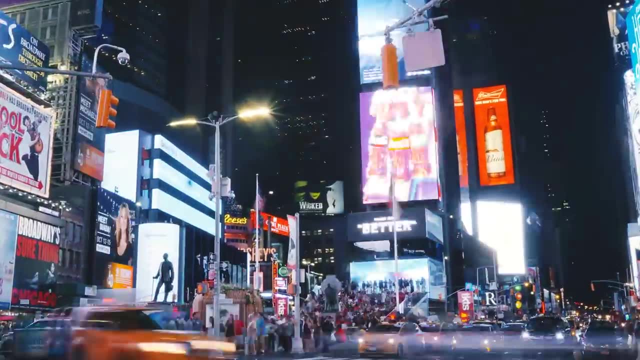 other pursuits before the next big thing or trend is announced. one must always be improving and always innovating, And what many companies must be doing now just to survive and thrive, is be as flashy, click-baity and fast as possible, no matter how objectively true their 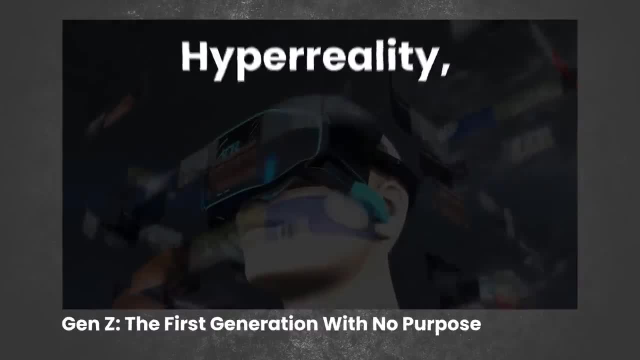 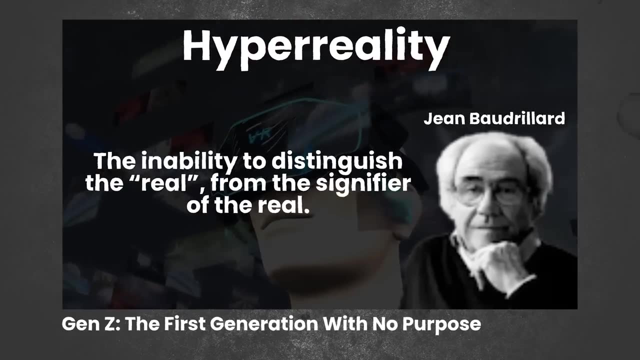 statements are. In my video on Gen Z's lack of purpose, I talked about the idea of hyper-reality, which essentially means that the online world starts to become indistinguishable from the things in the real world it's trying to represent, And the part of hyper-reality that is being brought upon by click-bait and controversy. 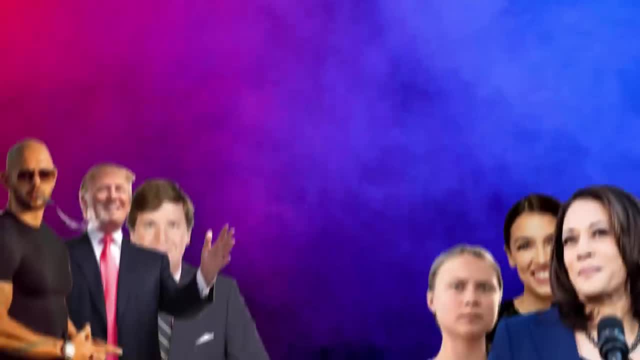 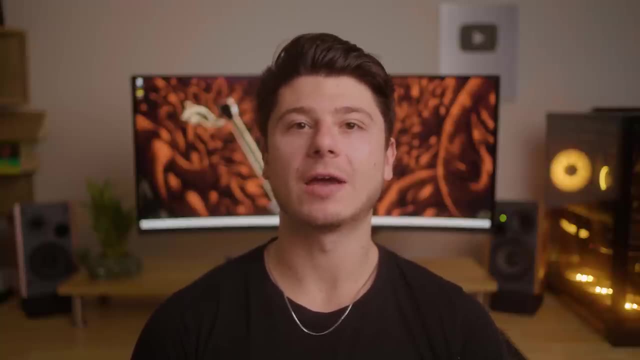 that is now affecting everyone's critical thinking skills is the increase in polarization and superlatives. I want you to take a look at these video clips and see if you can figure out what they all have in common. In this video revealing the laziest way to make money online, 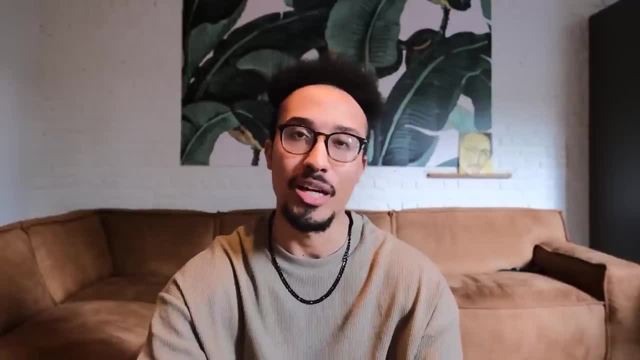 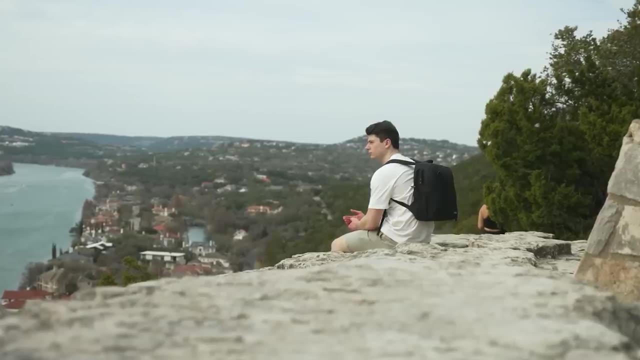 The worst advice you will ever hear in this chair: How to learn a language as fast as humanly possible. She's the worst mayor in America right now. The most important factor towards building the life you want: Did you pick up on it? 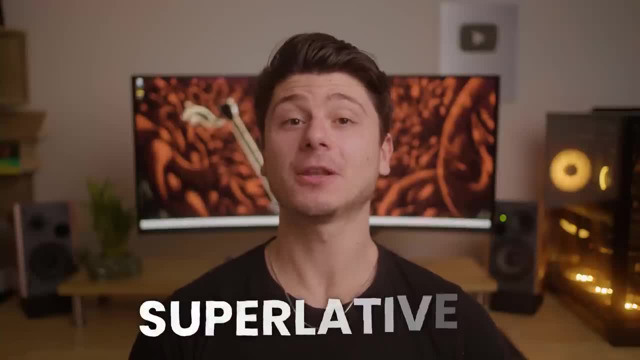 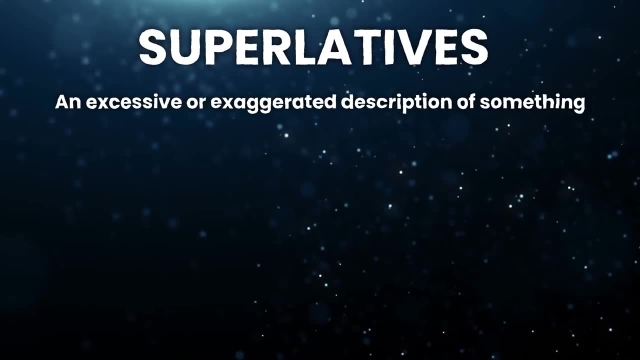 Well, if you didn't, it's that every single person in these clips used superlatives to describe what they were talking about. A superlative is an exaggerated or excessive adjective used to describe something: The absolute worst, the best, the biggest, the smallest. I hate, I love. 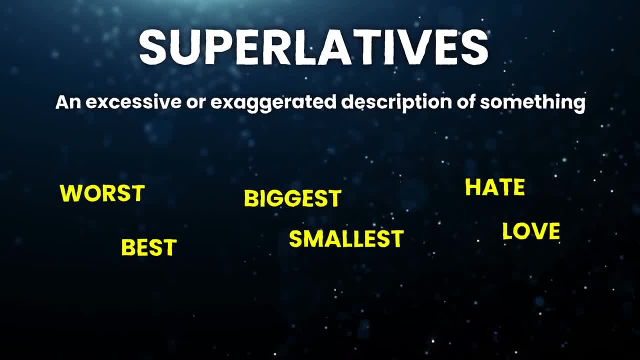 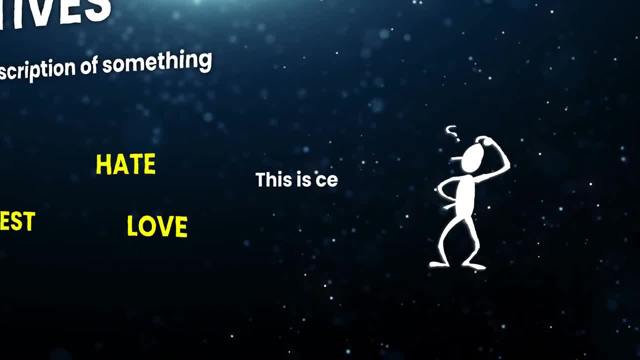 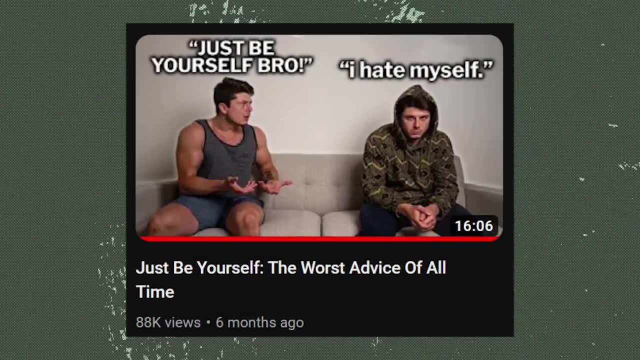 And when things are labeled as the best, worst, fastest or slowest, it gives people no space to wonder if there might be some information related to what you're consuming that is better out there. In other words, people would much rather click or read something that says the worst advice. 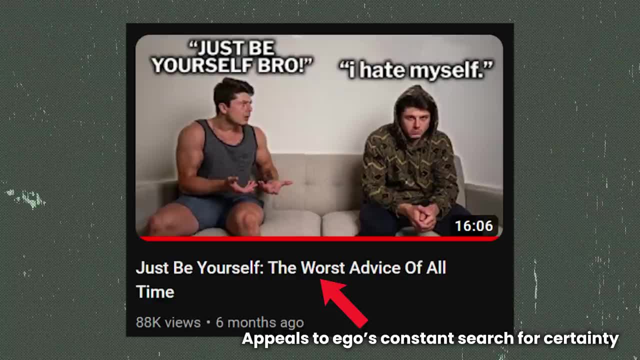 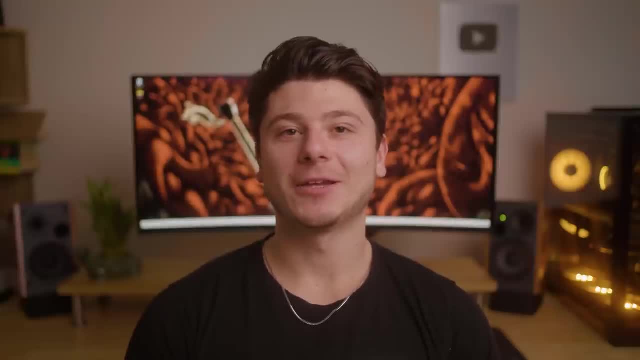 of all time rather than the advice. that's very bad because it leaves no room for doubt and scepticism and appeals to our egos' constant search for certainty. And yes, I am using one of my videos as an example here to show you that I have to play. 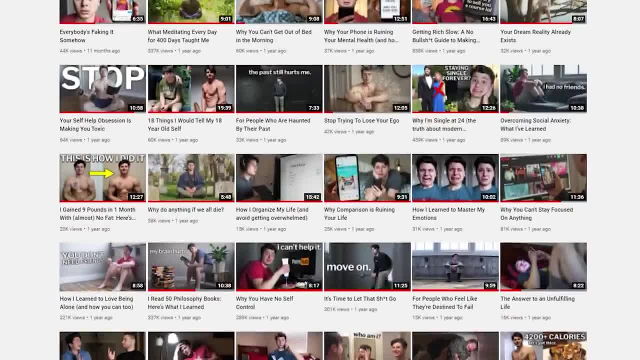 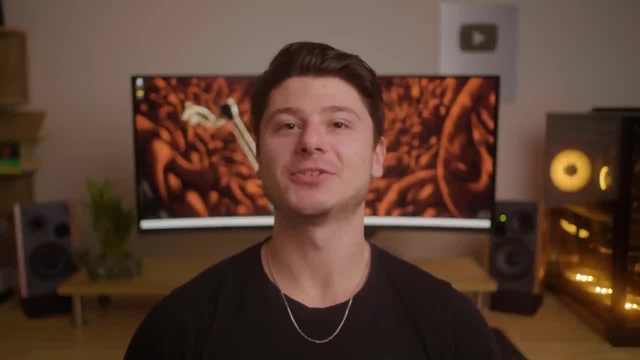 this game of polar czys. in my titles and thumbnails too, say that everything I present in my videos, once you get past the clickbait title and thumbnail, is nuanced information, and that is the way I will always present information. But for many 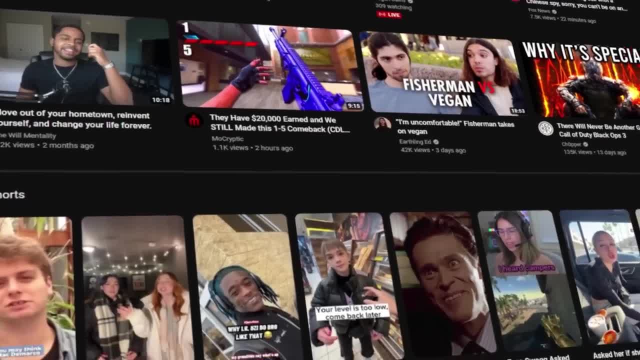 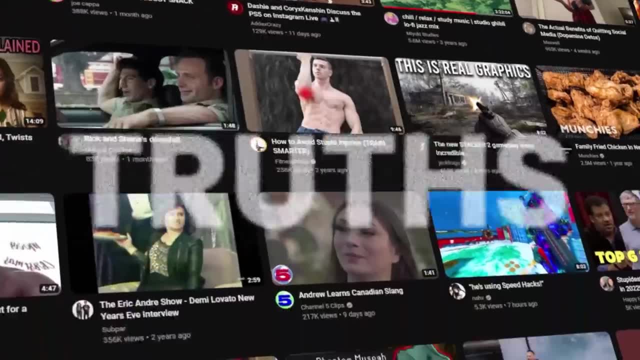 cases online, people aren't doing this. Hyper-competitiveness has pushed us to a state in which people are promoting incomplete, sometimes inaccurate, opinions and ideas disguised as absolute truth just so they can retain their relevancy. In other words, misinformation is being 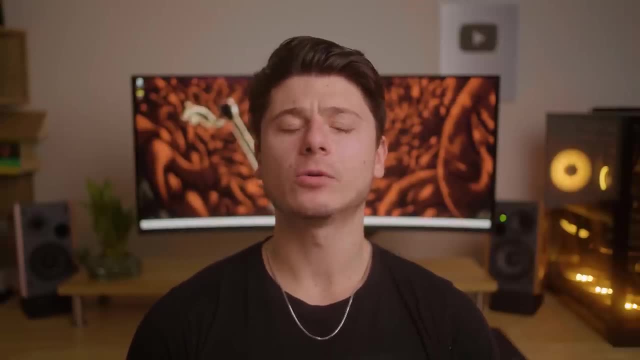 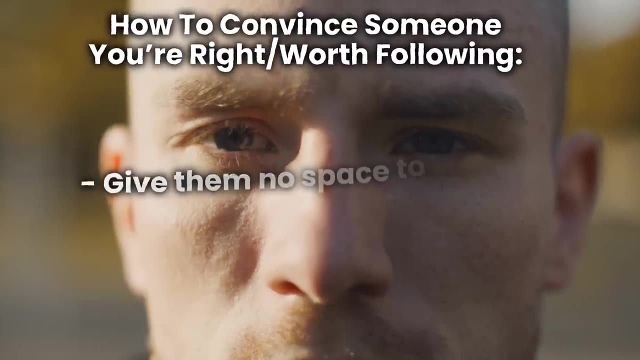 spread ever more rapidly, just so people can get the bag. Now let me ask you a question: What's the easiest way to convince someone you are right and worth following? Well, in my experience, you just need to give them no space to question your stance. speak with confidence and conviction. 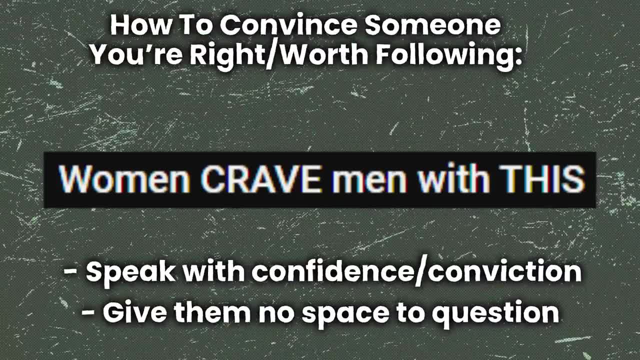 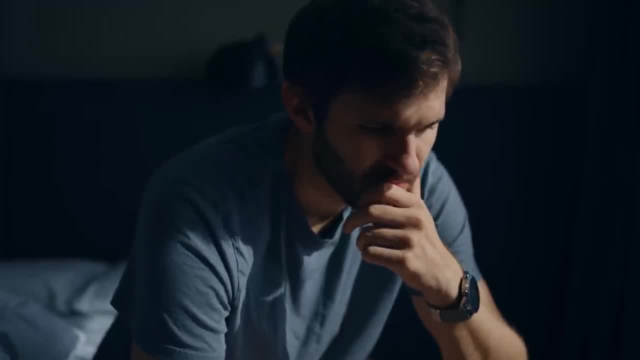 and title everything and say everything with those superlatives that we talked about earlier. This type of devotion to one person isn't new. it's been prominent throughout history, Because life without guidance, meaning and certainty is extremely anxiety-inducing. After all, you are. 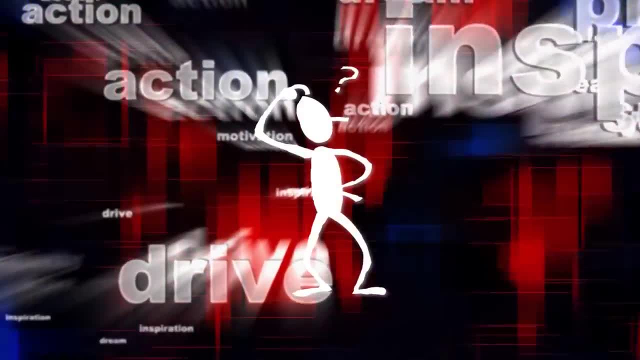 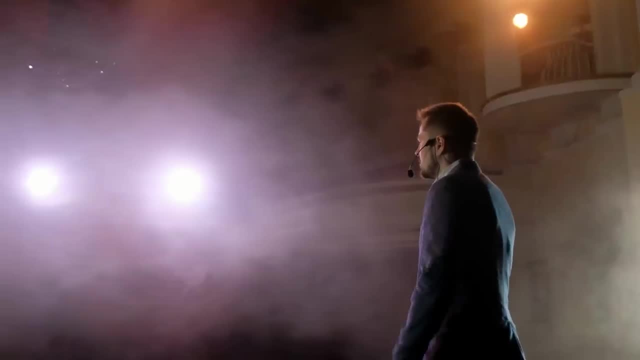 spawned into a world you have no previous knowledge on, and you are supposed to figure out what to do with this unlimited freedom of thought. For most people, the idea of that is too much to bear, And so, naturally, people turn to the leaders, aka the people that seem to have everything figured out and have all the answers. 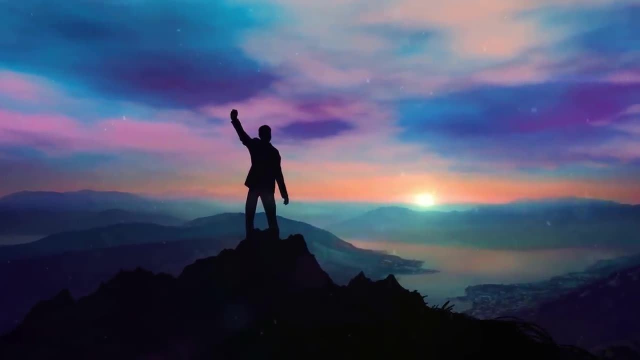 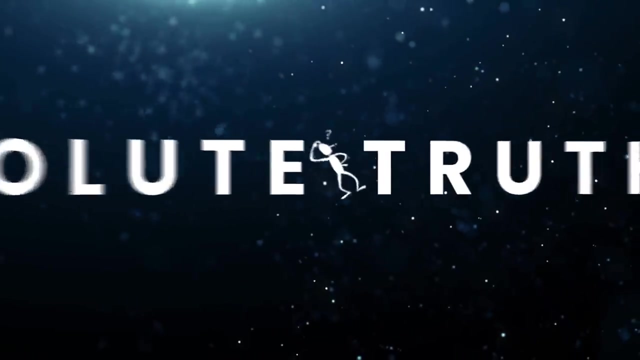 Because at least then they have something to believe in and a direction to strive towards. But the one person you should be wary of more than anything is the person who claims to have the absolute truth about everything they talk about and they give you no space to question. 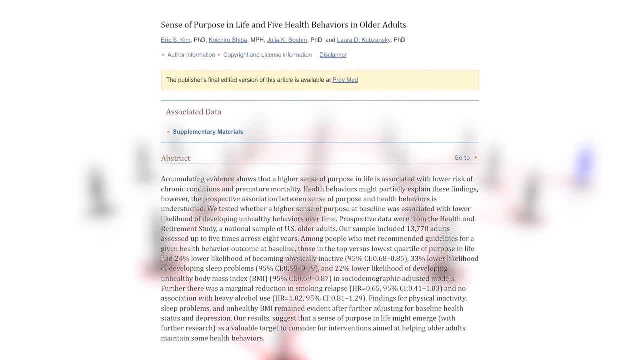 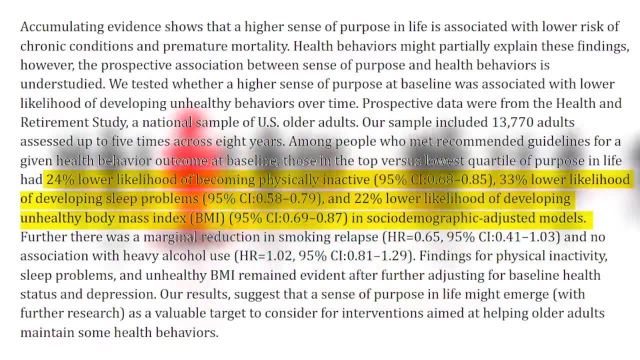 them or think for yourself. Now I will say: the people with meaning and direction in their lives do tend to live much happier, healthier lives than those with absolutely no meaning. And we need leaders because at the very least, they give us strength and help to give us some sense of the 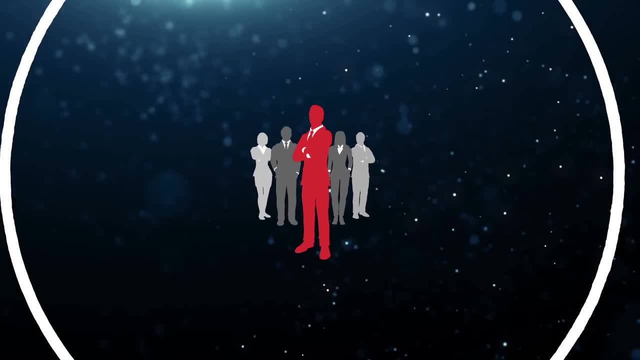 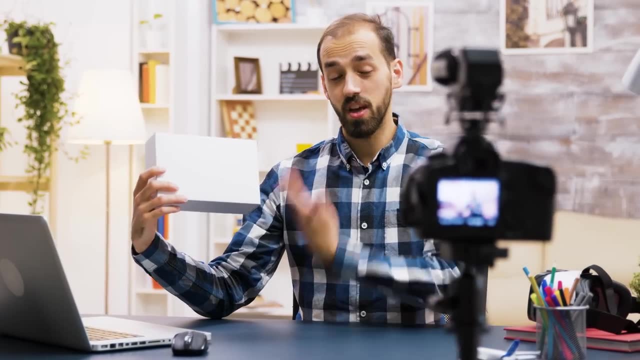 world. But the problem arises when you completely lose your ability to see outside of that bubble or leader that has given you that certainty, meaning and direction, And since almost anyone with an internet connection, some confidence and a general understanding of human psychology can, 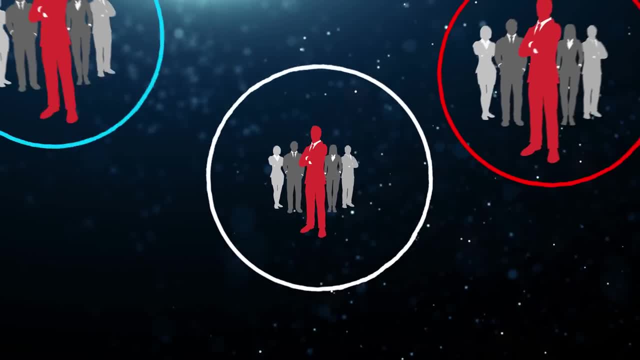 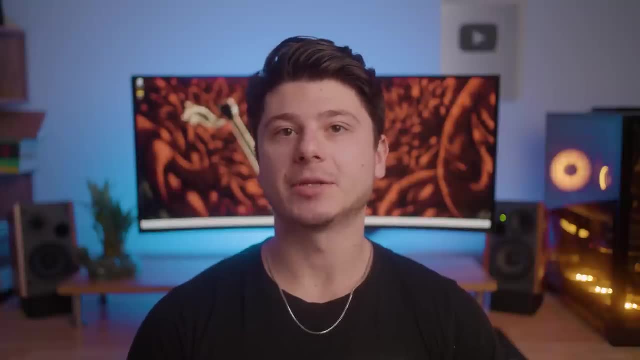 amass a following: now there are tons of new, different bubbles with different gurus that all seem to have the same purpose, And so if you are a leader, you are a leader, And if you are a leader, you are a leader. And this is where a very dangerous thing starts to happen, which is: 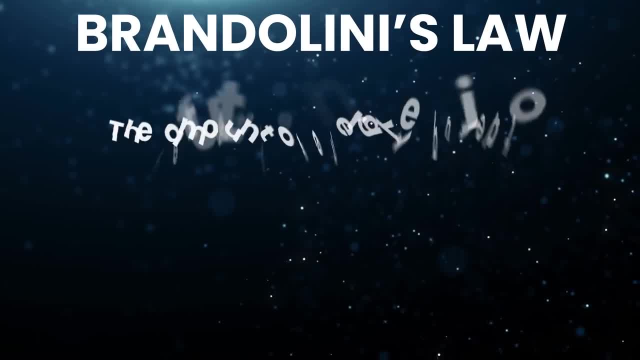 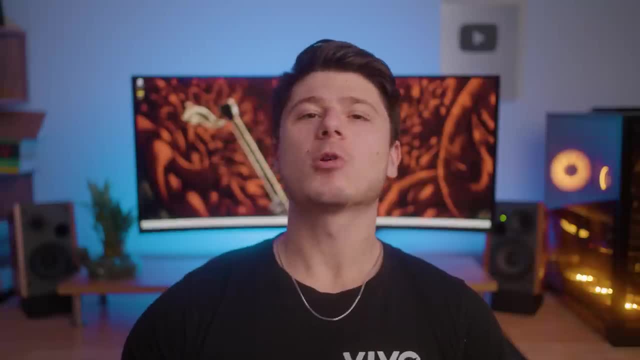 referred to as Brandolini's Law. This law states that the amount of energy required to refute bulls**t on the internet is an order of magnitude greater than it takes to produce it. In other words, it takes way more cognitive energy to question the information that you are presented. 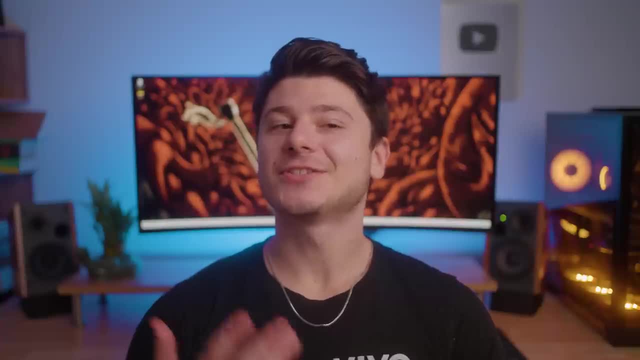 with online rather than to just accept it as truth. And since most people think like a bot, they're just going to take whatever is presented to them the most as truth and, in turn, that is going to make misinformation so hard to understand. And so if you are a leader, you are a leader. 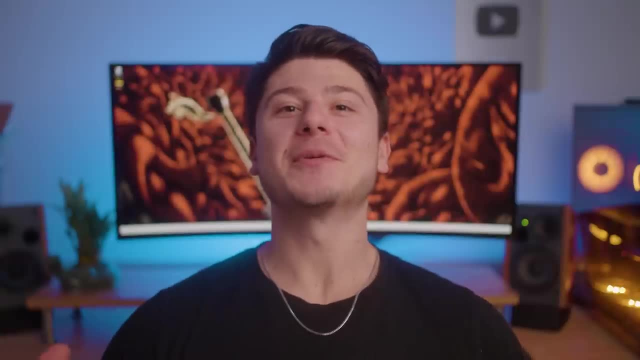 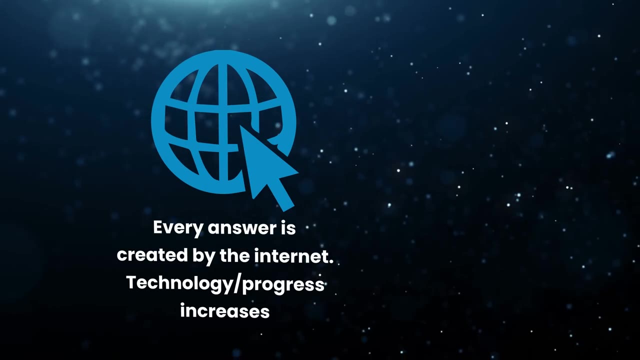 So this is where everything we've been talking about so far starts to pile up. The internet has created every type of answer you can think of, and the technology behind it has made progress speed up exponentially. Because of that speed and extreme obsession with improvement, we are now 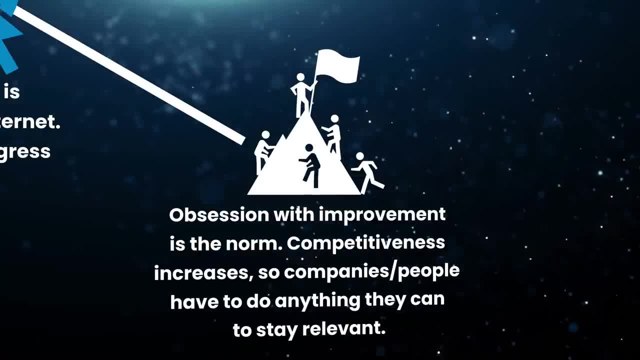 seeing companies are forced to be ultra-competitive, to the point where they have less time to think about their decisions and instead just keep up with the times, And because of this our society has become much less accepting of average. So the only way most of these companies or any prominent 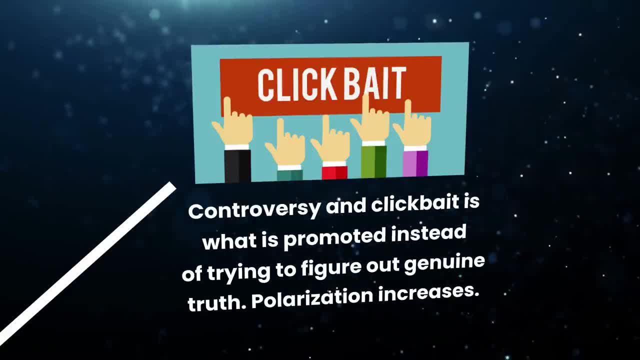 voice on the internet can stand out and beat the competition is to be as polarizing, flashy and controversial as possible, even if nothing they do or say is for the greater good or has some objective, rational truth behind it. Therefore, echo chambers, or bubbles as I like to call them, 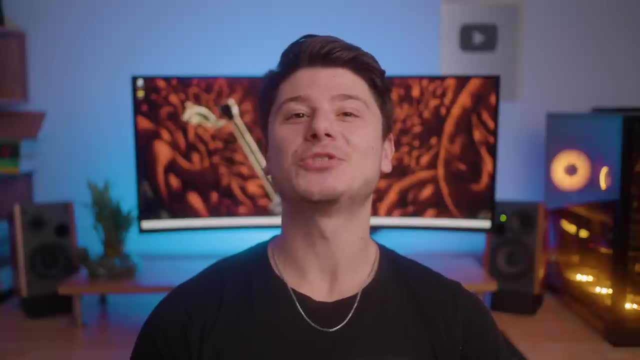 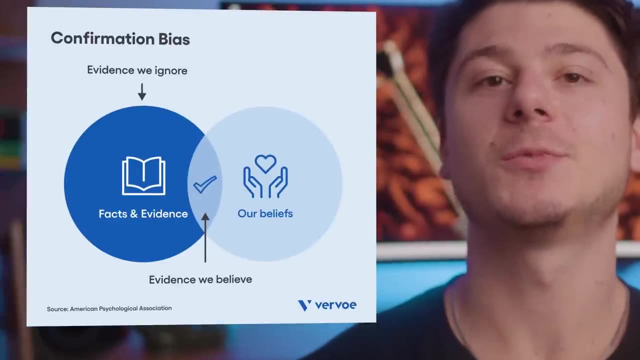 have now become the norm. And what happens when every echo chamber you can think of exists? Well, it means it's much easier for people to not think critically and simply resort to confirmation bias, which is our tendency to look for information that validates our already. 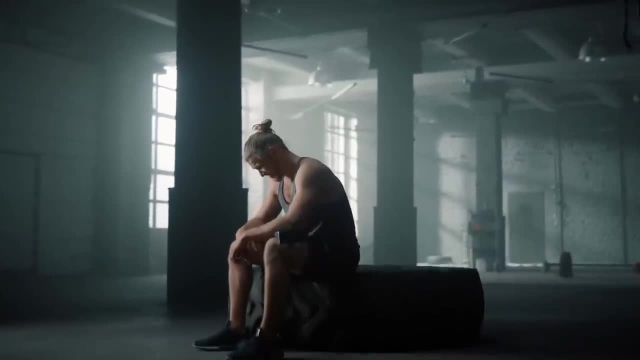 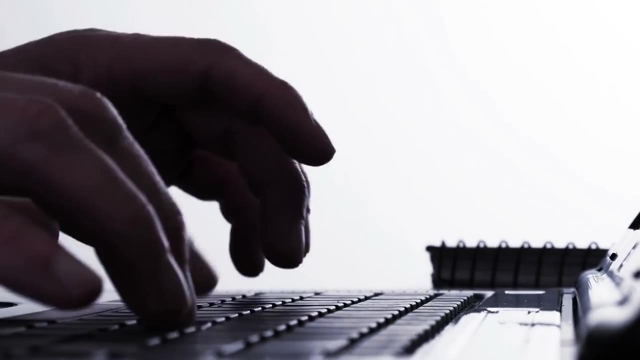 existing beliefs. For example, when one gets traumatized by a woman they fall in love with and they start to think all women are untrustworthy, they may end up going to the internet to see if other guys have experienced something similar, And that in turn could lead. 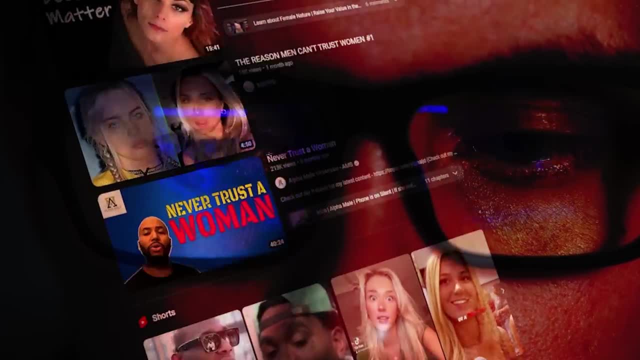 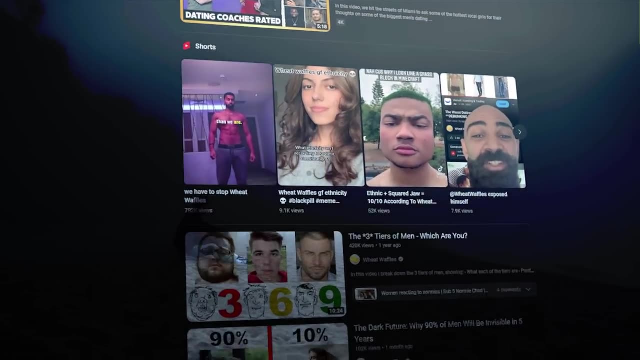 them down the red pill rabbit hole and have them only consuming red pill content that aligns with their biases. Or if one has always gotten rejected by women, they might turn to the black pill bubble and start believing looks and height are the only things that matter when it comes to getting a girl. 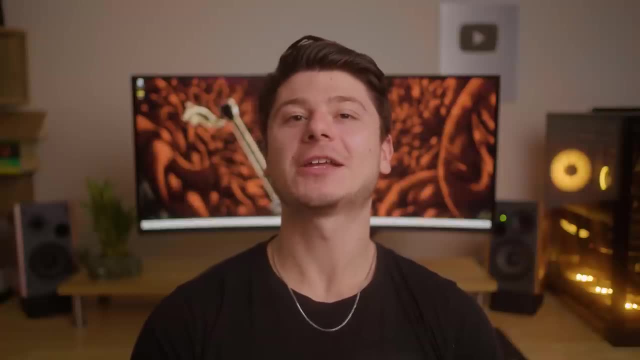 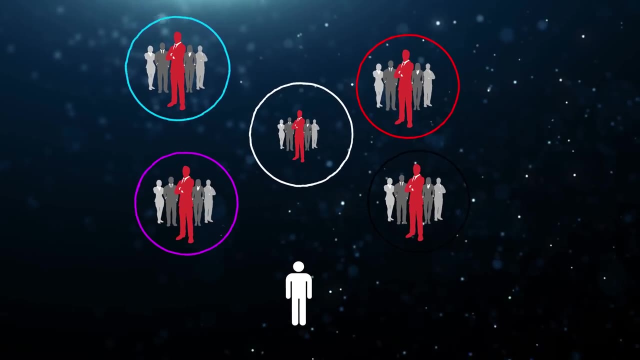 to like you, No matter how biased your opinions are. there's sure to be an internet community that is spewing your already biased beliefs as absolute truths. Red pill, black pill, purple pill, liberals, conservatives- all of these communities and political groups can help an NPC or bot with a. 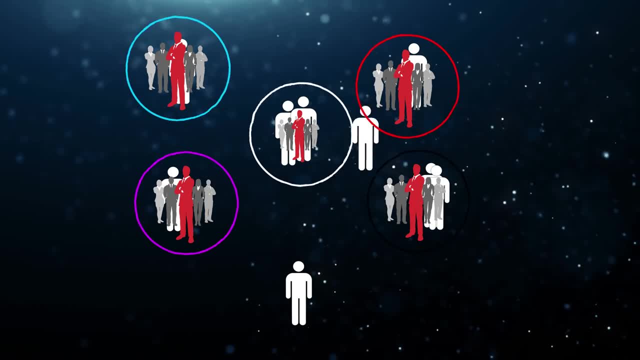 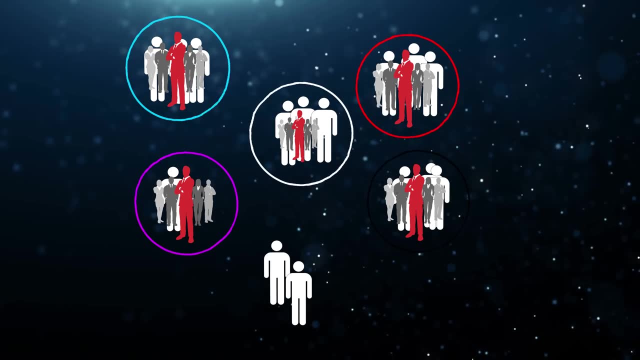 serious lack of critical thinking skills, fall into the trap of thinking their life experiences that created the biases they have is the only way the world actually is and that their solutions are the only right solutions, When the truth is that all of these communities that are clashing with one 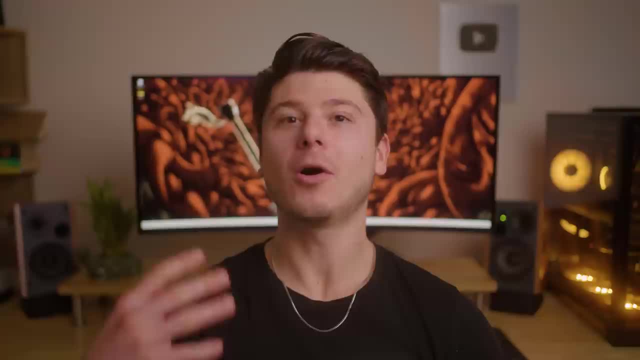 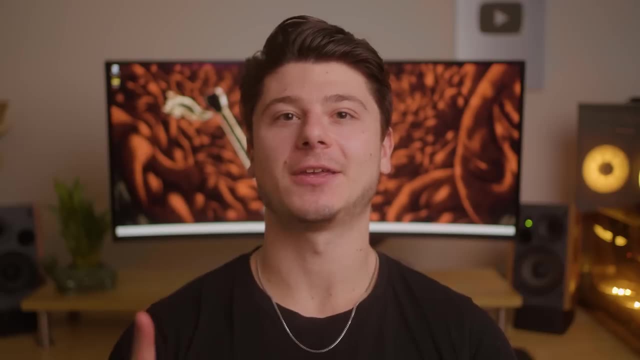 another. they all have a certain bit of truth to their beliefs. they all have a certain bit of truth to them and they all spit a certain bit of objective truth. But not one community itself has the objective, right answer to everything. This problem is only further exacerbated by social 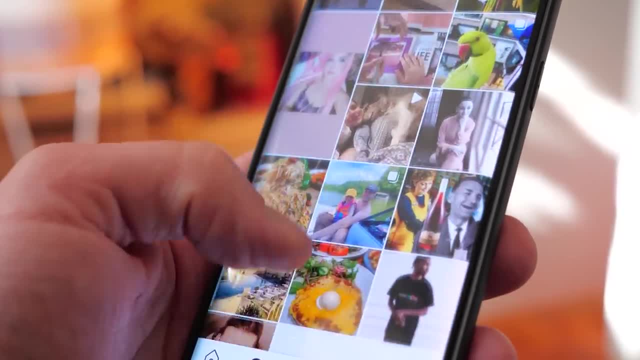 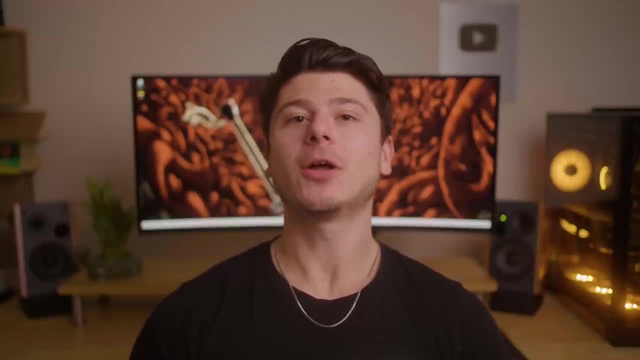 media algorithms which will show you things you have already been searching for, following and watching. So, instead of using the internet as a way to broaden their view on the world and become more open-minded, most people are just picking and choosing the information that best. 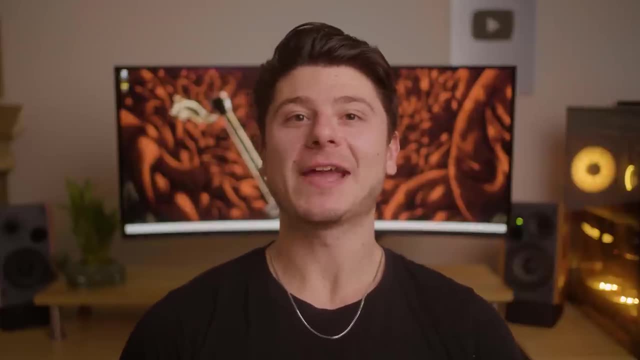 suits their echo chamber of subjective truths, And this is why I think everybody seems to disagree with or hate every single one of these things. And I think this is why I think everybody seems to disagree with or hate every single one of these things, And this is why I think everybody seems to 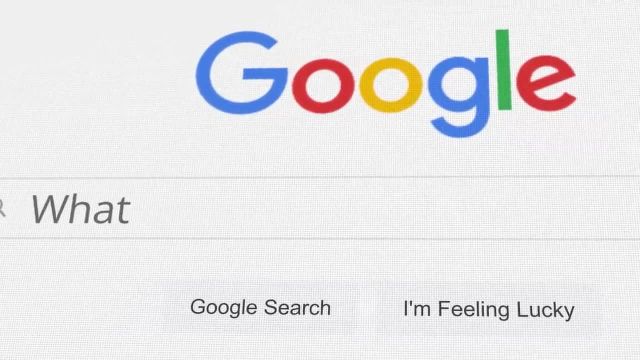 disagree with or hate every single one of these things, And this is why I think everybody seems to disagree with or hate everyone else now, Not just because there are so many different opinions on what is true or not, but also because it seems like the validity of one's bubble they find themselves. 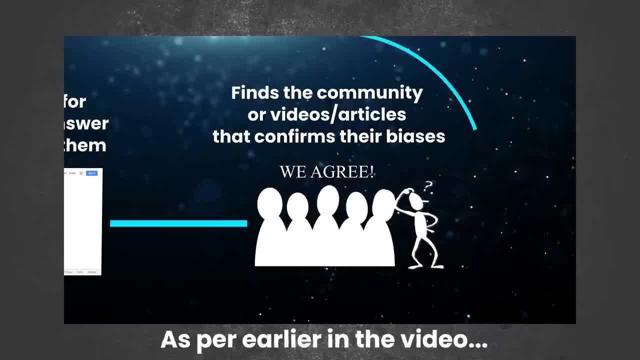 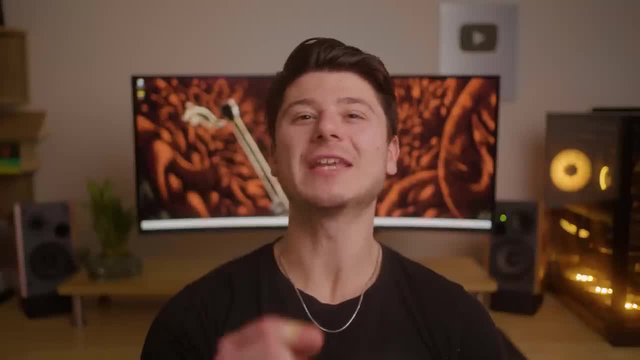 trapped in is so much stronger due to how many more people are giving them social confirmation online. The divide between humans feels stronger than ever, and it feels like if you have just one different opinion than someone, they will immediately label you as wrong or a bad person. 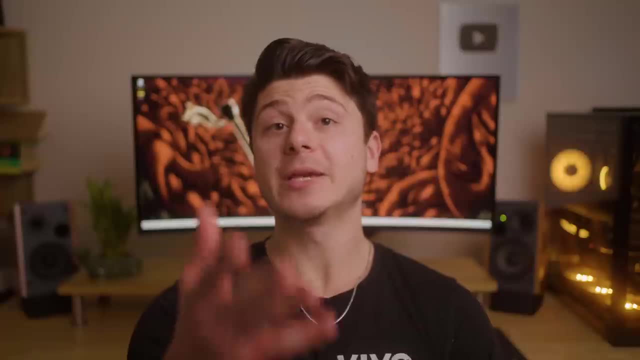 So now that we have a better understanding of how a lot of people- and maybe you- lack in critical thinking skills, they will immediately label you as wrong or a bad person. So, now that we have a better understanding of how a lot of people, and maybe you- lack in critical thinking skills, we must now 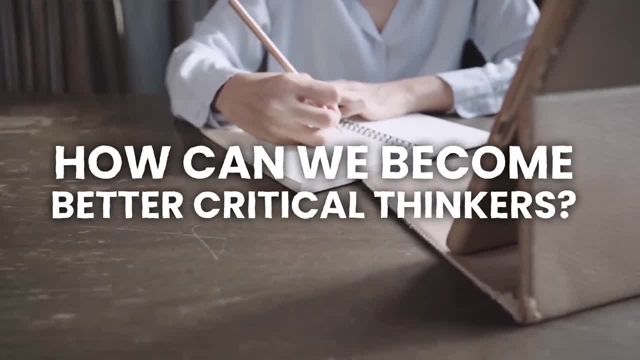 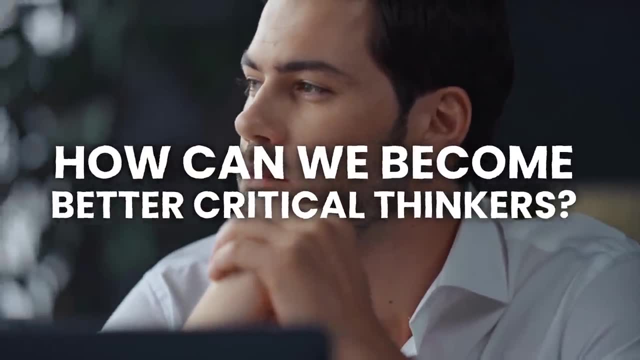 ask this question: How can each one of us become better critical thinkers and not be so inclined to instantly believe or look for information that confirms our biases? Well, in order to do so, we first need to understand the two systems of thinking that our brain usually uses. that I've. 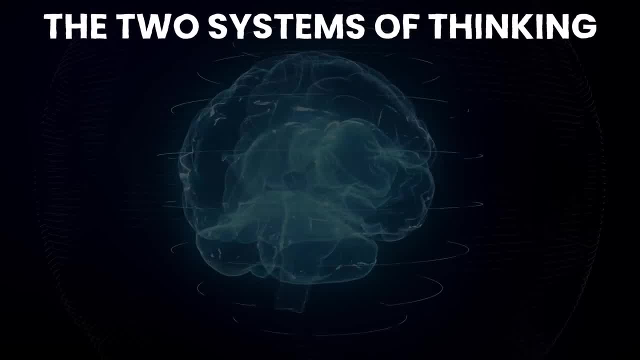 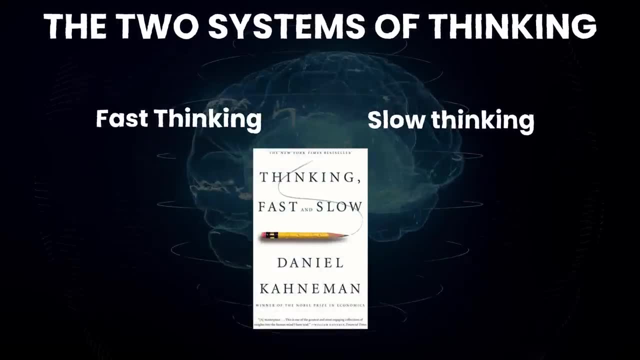 been referencing throughout this video. The two systems of thinking that we typically use are called fast thinking and slow thinking, and these terms were popularized by the book Thinking Fast and Slow by Daniel Kahneman, and the book is called Fast Thinking and Slow Thinking, and these terms 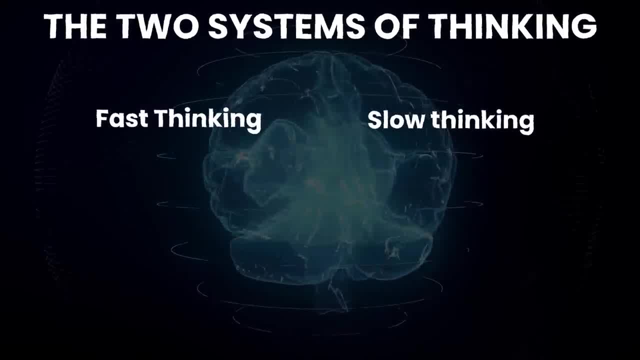 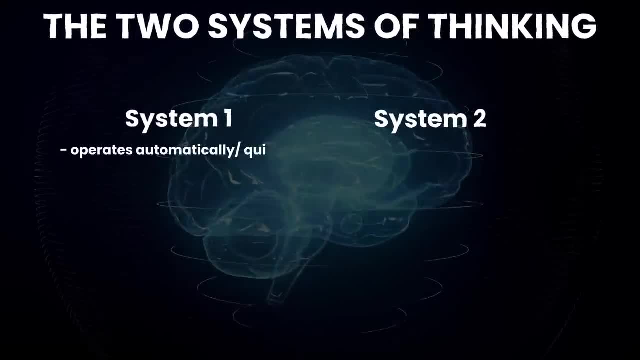 were popularized by the book Thinking Fast and Slow and Daniel Kahneman. And like Kahneman does in the book, we're going to refer to fast thinking as system one thinking and slow thinking as system two thinking. Our system one of thinking operates automatically and quickly with little to no effort. 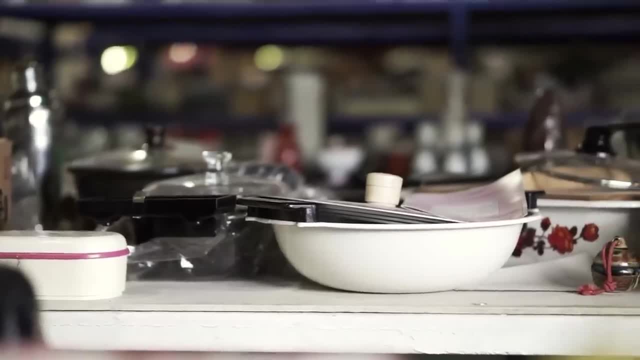 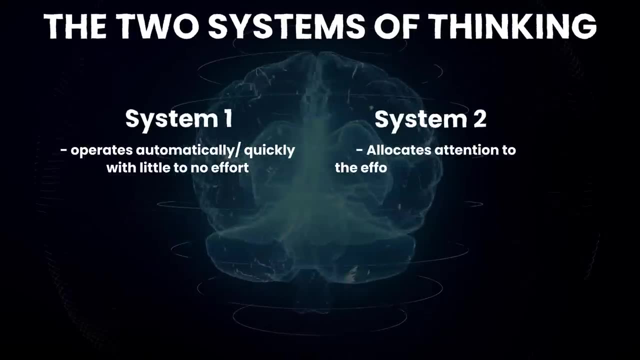 and no sense of voluntary control. Examples of this are detecting that one object is farther than another, reading a simple sentence or driving a car on an empty road. The system two of thinking allocates attention to the effortful mental activities that demand it. 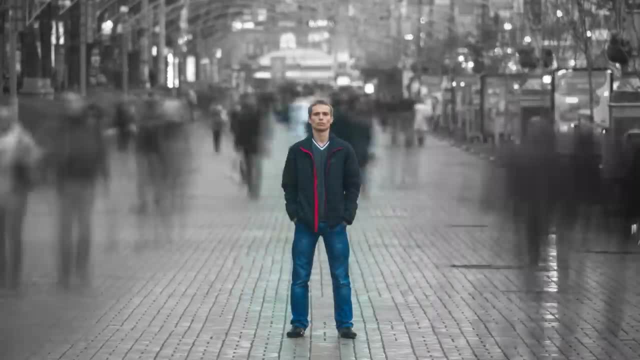 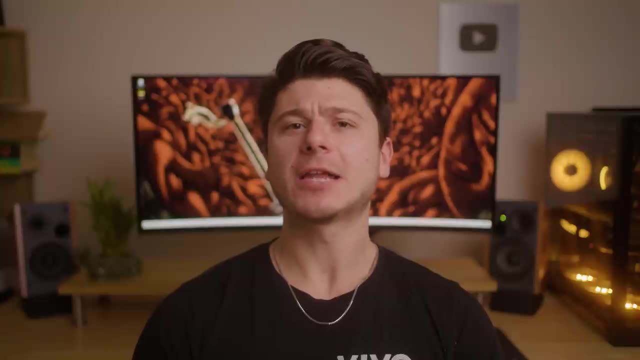 Examples of system two thinking are focusing your attention on a particular person in a crowd exercising faster than is normal for you or, as it relates to this video, thinking critically, If we want to stop letting our biases, triggers and closed-minded worldviews 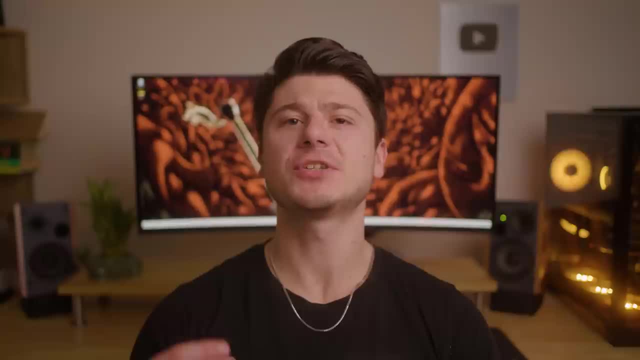 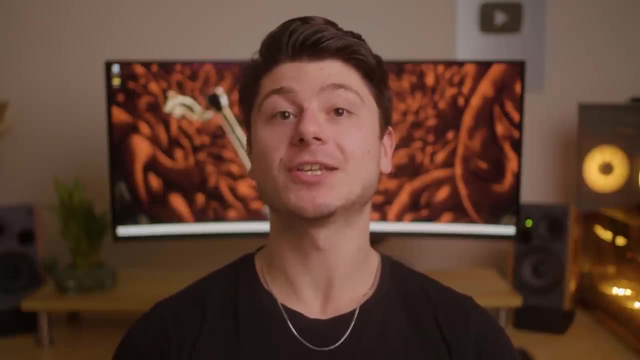 govern all of our actions, then we must learn how to use our system two, thinking more, and how to use it properly. And I say properly because it's very easy to have a lazy system two that doesn't actually do the critical thinking work, especially given our modern information age. 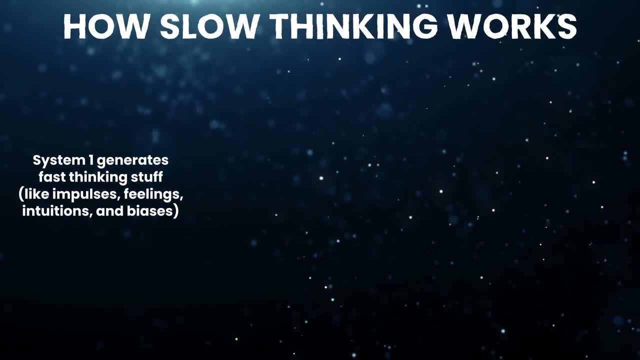 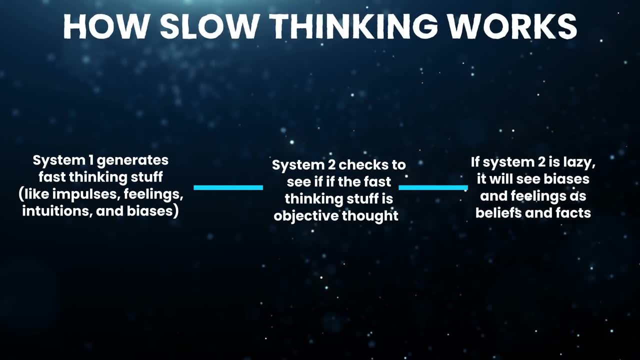 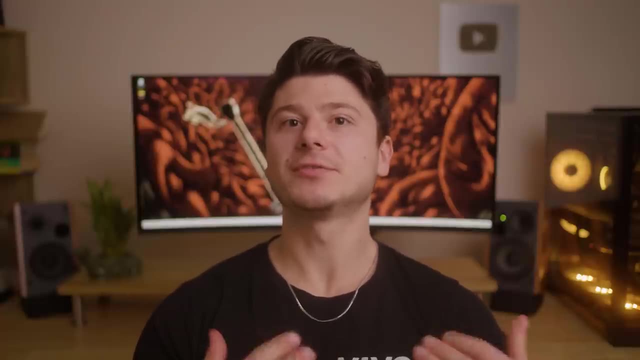 You see, system one automatically generates suggestions, feelings and intuition and if endorsed by a lazy system two, intuitions end up turning into beliefs and impulses turn into voluntary actions. So, basically, if you have a very lazy, improper system two, it will accept the faults of system one and not question them, and just. 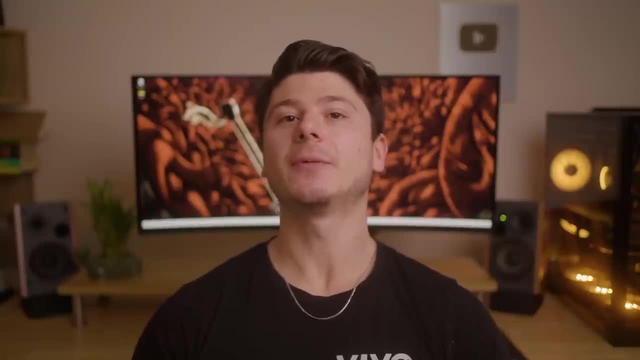 believe them as fact, which will then lead to you developing those cognitive biases that we talked about earlier, and, most notably, confirmation bias. So the next time you're watching someone or you're presented with a question, take a quick pause and ask yourself. 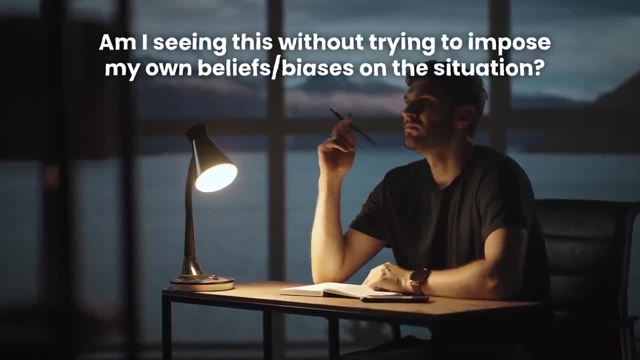 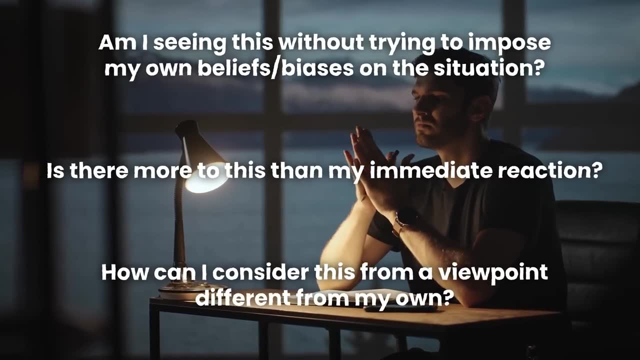 Am I seeing this without trying to impose my own beliefs and biases on the situation? Is there more to this than my immediate reaction, And how can I consider this from a viewpoint different from my own? Pay attention to how your body and mind is reacting and how it is. 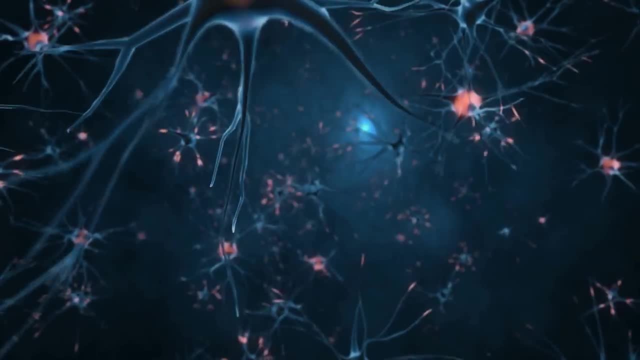 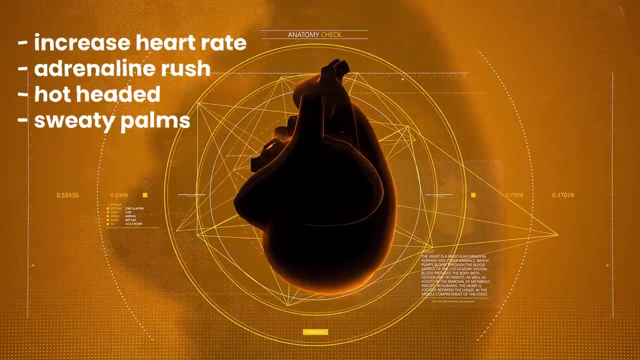 simply a process of the ego not being able to come to terms with potentially being wrong. This usually presents itself as an increased heart rate, an adrenaline rush, racing thoughts and sweaty palms. To manage the stress of a decision or piece of content, go for a quick walk. 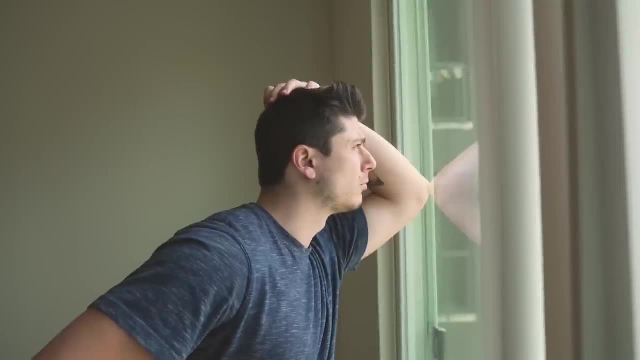 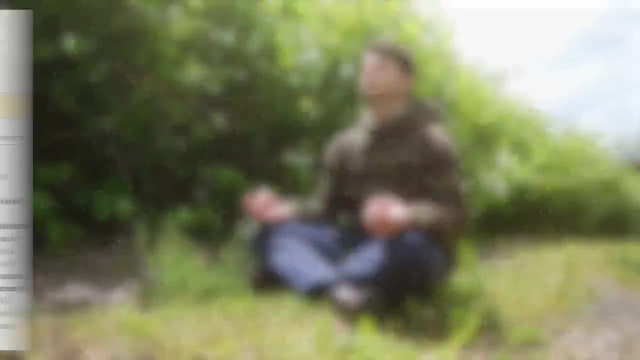 or reassessing what has been presented to you, Take prolonged periods to do simply nothing but stare at a wall. And, as I've said before and I'll keep saying again: meditate, Mindfulness. meditation helps your system two to not be so lazy and will help you to be more objective when 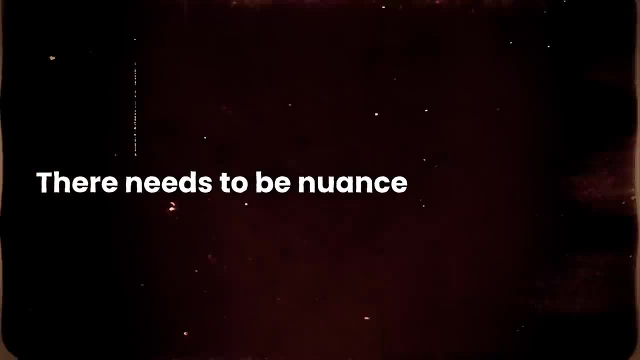 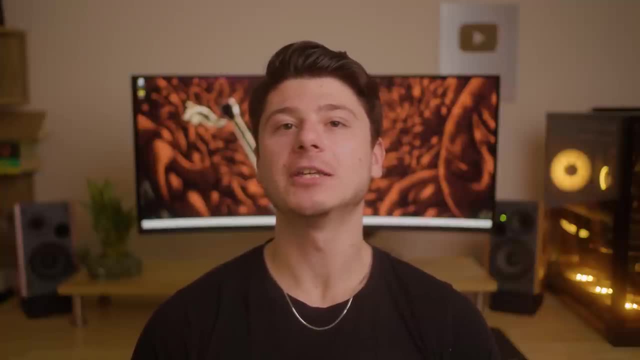 the time is right Now. as I always say, there needs to be nuance, even with nuance itself. If you are always trying to think critically about all your decisions, actions and thoughts, then that will lead you to overthink and just do more harm than good. 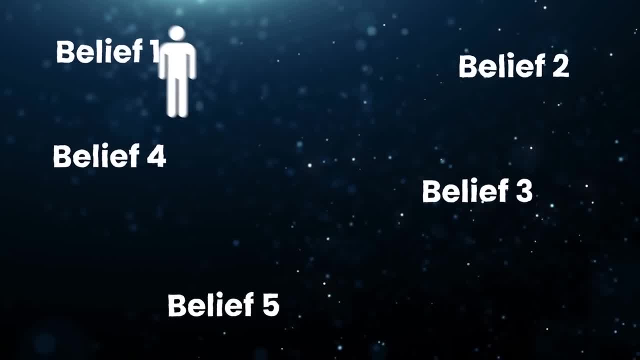 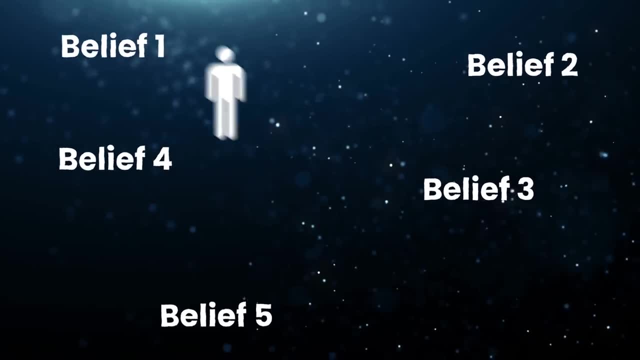 If you don't stand for anything and you let anyone's opinion overtake your current one, you're simply a human pinballer bouncing around one belief to another, and you are far more easily taken advantage of and less respected, Because nobody likes a people pleaser who agrees with. 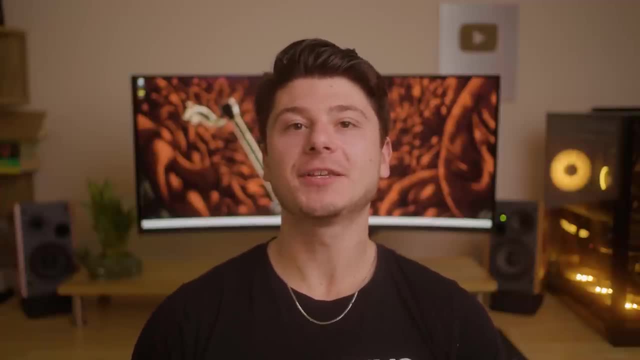 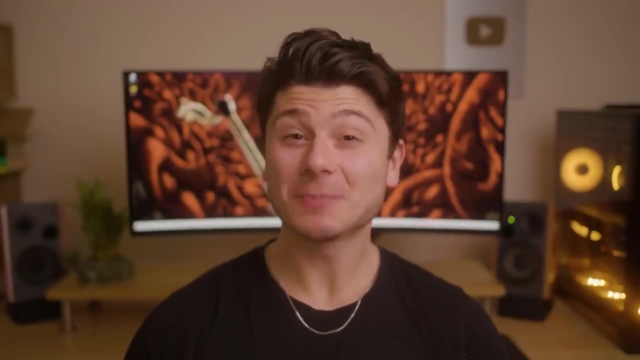 everything everyone says The reason you want to hone your system, two thinking skills- isn't so you can be completely agreeable all the time. it's so you can become more open-minded to the possibility that maybe, just maybe, you're wrong and that there's more variables and experiences you need. 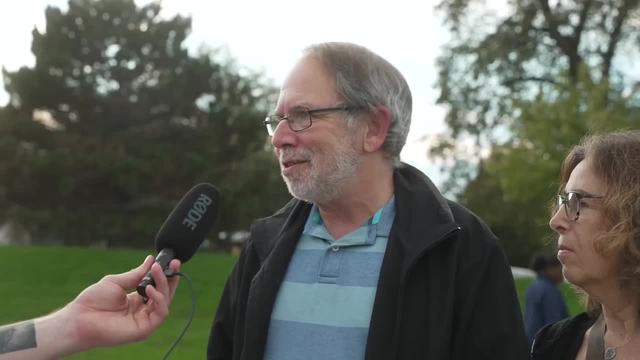 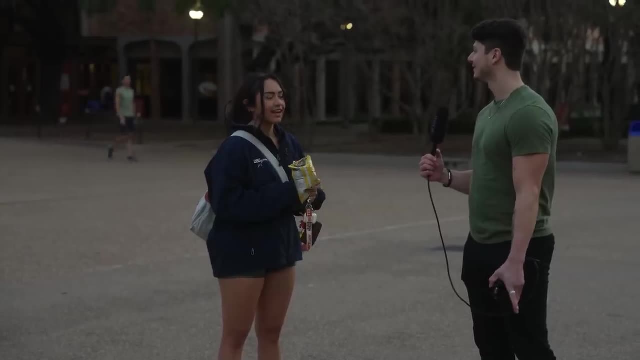 to have in order to form an objective picture, And it's about being more proactive instead of reactive, so we can all be open to more conscious, unbiased conversations that fuel progress. Now there is so much I left out from that book: Thinking Fast and Slow by Daniel Kahneman. 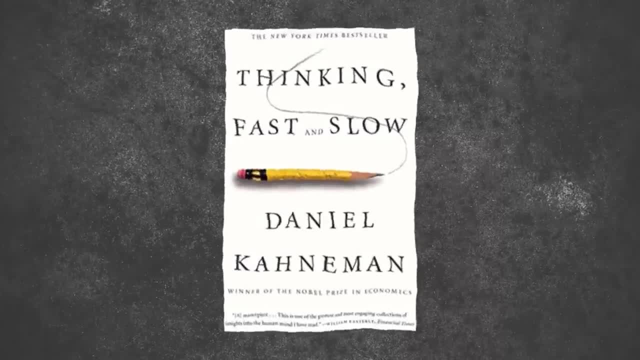 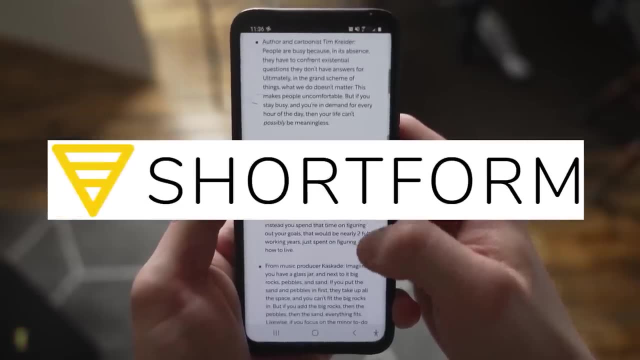 and it really is one of the best books to teach you how to become a better critical thinker. So if you're looking for a full, detailed summary on that book, I suggest you use the app Shortform, which is the sponsor of today's video. If you aren't familiar with Shortform, it is a platform. 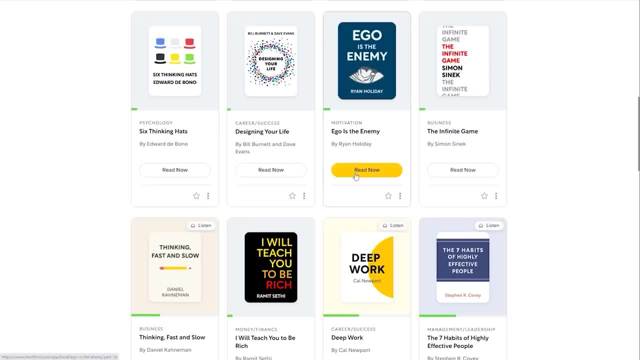 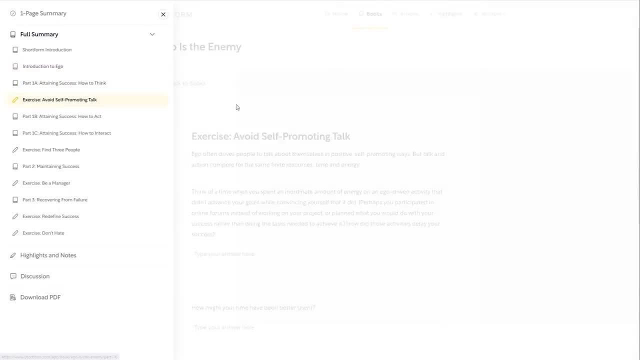 that is, producing high quality. high quality content that is free to use anywhere, anywhere. high quality guides to nonfiction books. They provide all the book's key ideas and concepts, plus smart commentary and analysis, and they also allow you to do exercises with each summary, as 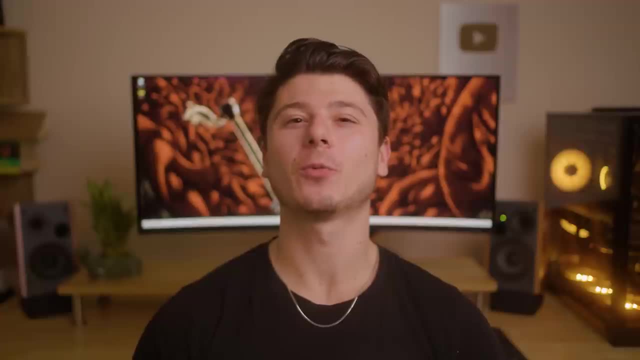 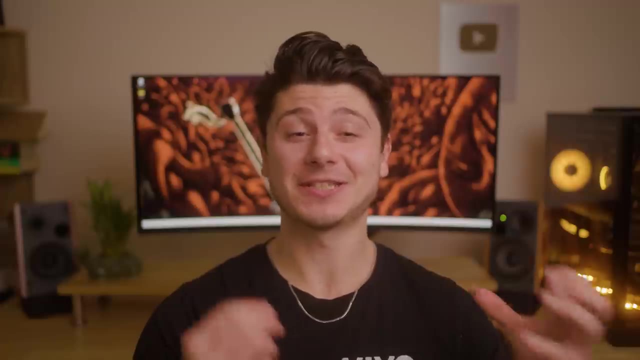 well, so you are directly applying what you've learned. And that's what I think really makes Shortform stand out above all these other book summary platforms is that you can actually apply what you're learning, and that, specifically, is super important to learning how to be a better 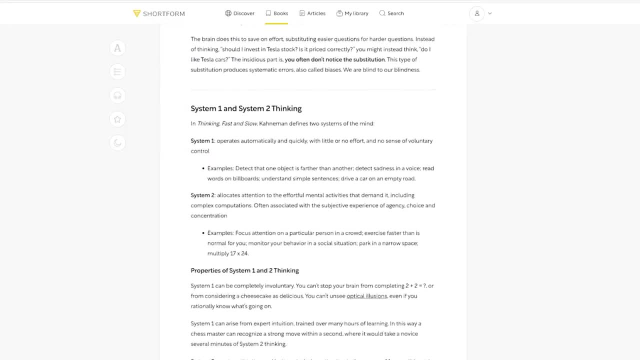 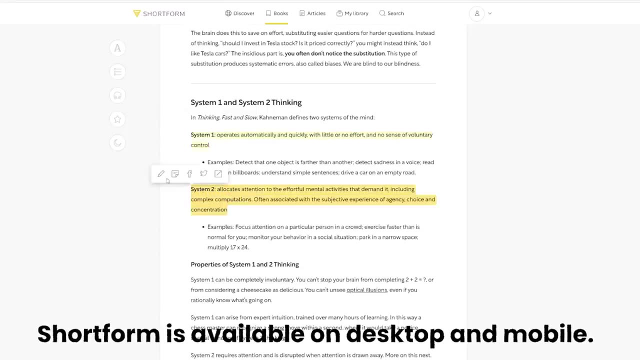 critical thinker. Like I said, I've gotten these ideas from Thinking Fast and Slow, but I got them. the short form summary that I read on there and the summary that they have for that book is excellent. Three genres I think you guys would really like are philosophy, psychology and self. 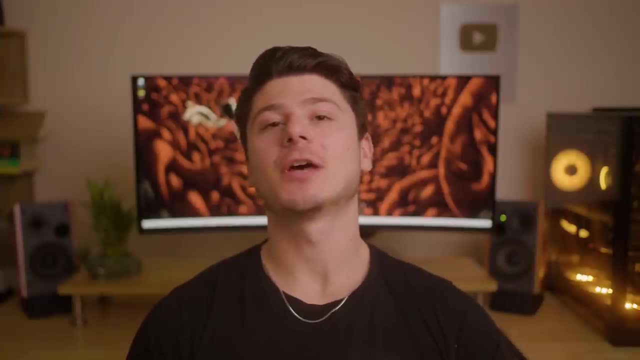 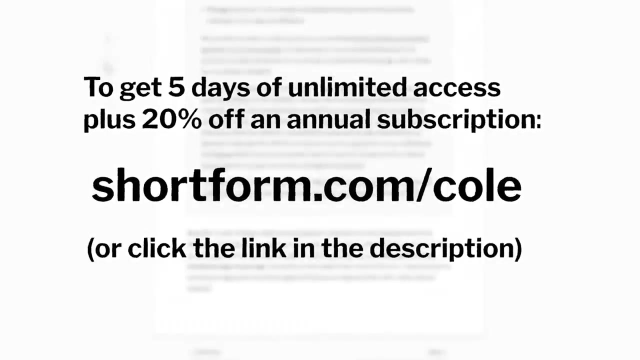 improvement. So if you're interested in reading that summary, along with thousands of other book summaries, for the price of just one book a month, you can go to the link in my description and that will give you five days of unlimited access, plus an additional 20% off their annual subscription. 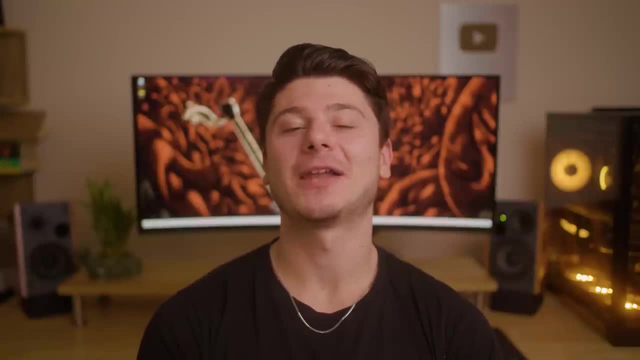 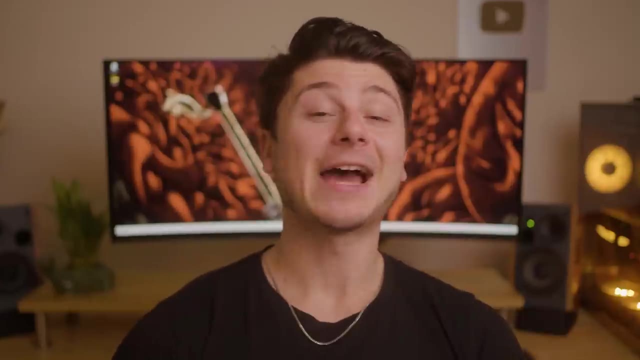 plan. So go, take advantage of that offer and check out my favorite book summary platform ever by going to shortformcom slash cole. The link to that, like I said, is in the description. Now, to help you become a better critical thinker, I want to give you your first critical thinking. 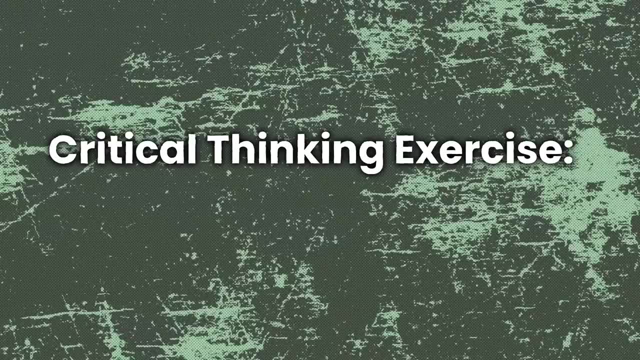 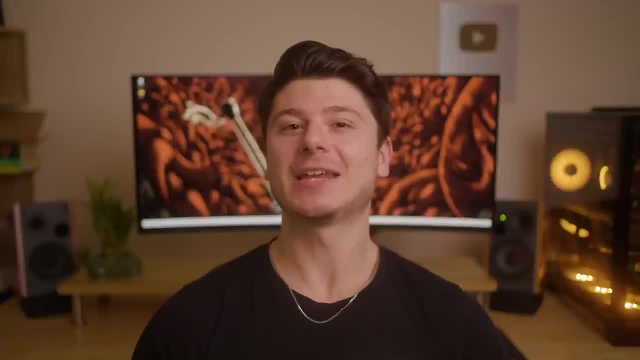 exercise. Think about what you've just watched in this video- and you can rewatch it if you need to- and tell me what you agree or disagree about what I said. When you're doing this, be sure to ask yourself if you're using any biases in your thinking and explain to me. 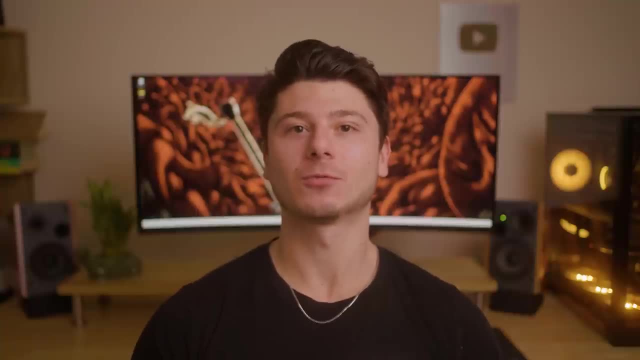 in the comments why you think what I said was wrong, using critical thinking. I look forward to a broader viewpoint on what I just talked about and sparking some useful conversations with you all. Thank you very much to all my patrons on Patreon If you don't know what this is. 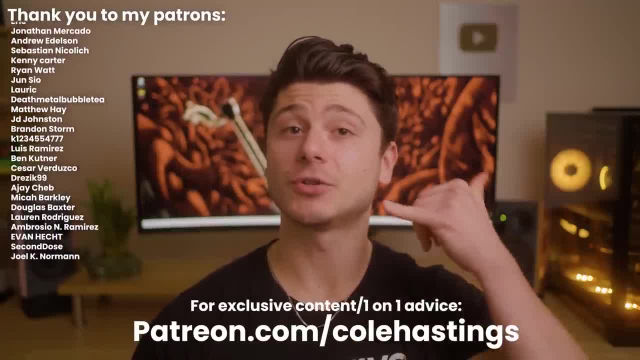 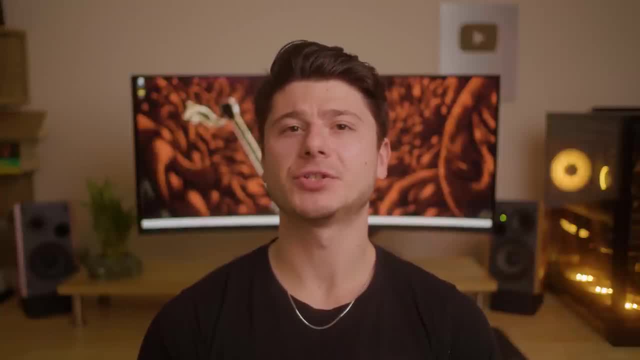 it's a platform separate from YouTube where I'm putting out exclusive content. You can also talk to me one-on-one over the phone on there. If you want to check that out- link in the description- And if you like these videos where I make video essays about modern issues going on right now and 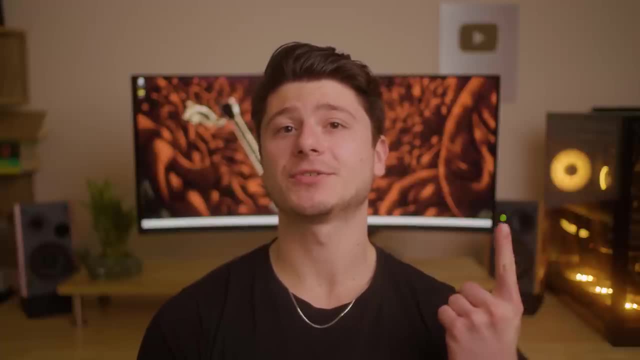 my potential solutions and how I feel about them. check out this playlist. I just made a whole playlist on all my video essays on modern issues, So if you're interested, yeah, go check them out. Maybe you'll enjoy them. And that is it. See you guys.